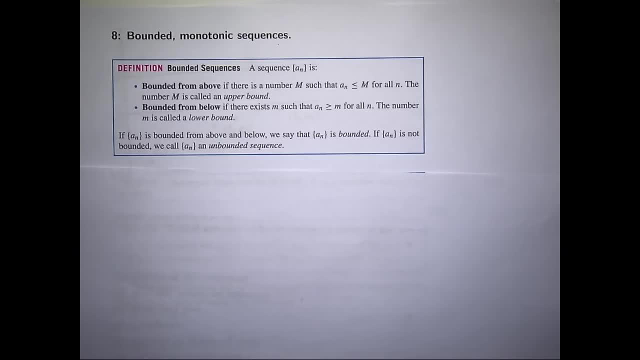 Alright, a few definitions. first, The definition involving a bounded sequence. well, I guess it involves two things really. We can bound a sequence in two ways: from above and from below. So we say that a sequence is bounded from above if there's. 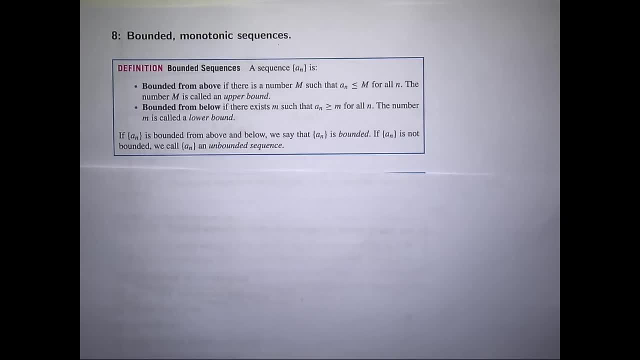 some number, big M, that the sequence is always less than or equal to. the value of the sequence is less than or equal to, Okay, and we call such a bound an upper bound. We can also talk about a sequence being bounded from below, where we just reverse the inequality sign. 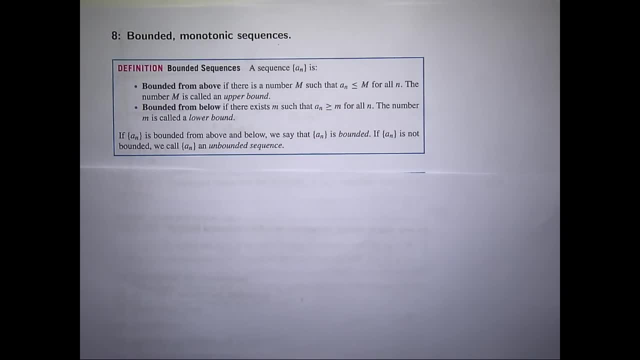 And we'll refer to little m as a lower bound. Now, if we have the situation where a sequence is bounded from above and below, then we call it a bounded sequence. So let me show you some examples to really give you an idea of what's going on here. 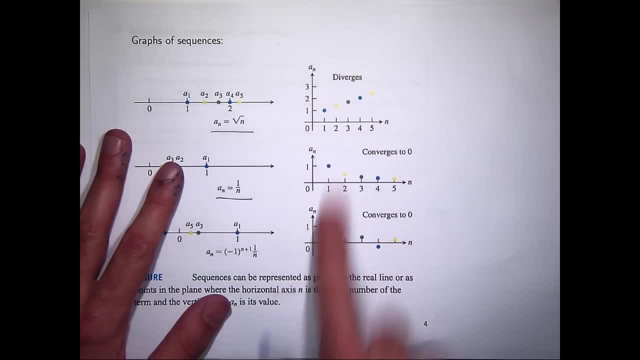 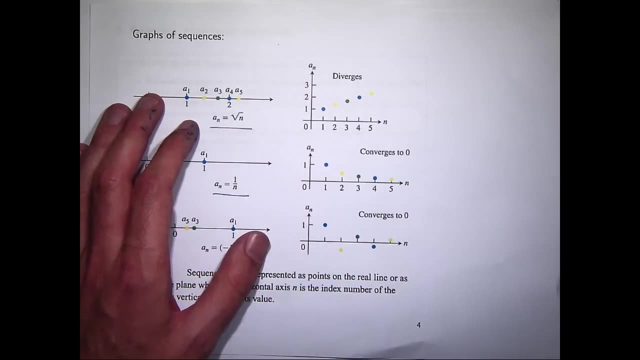 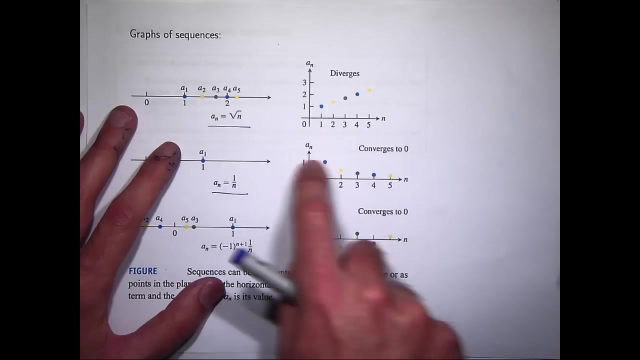 So just look at these three basic pictures here You can see for this particular sequence. the sequence looks like it's bounded below by positive 1.. Okay, but the sequence wouldn't be bounded above. In this graph the sequence is bounded above by positive 1, and below by 0.. 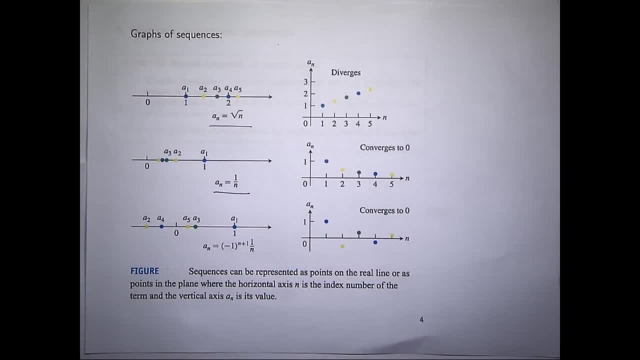 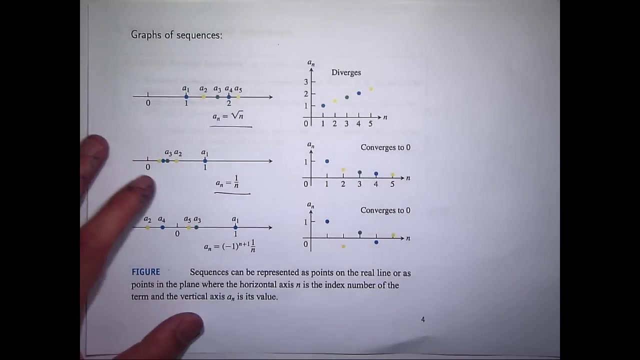 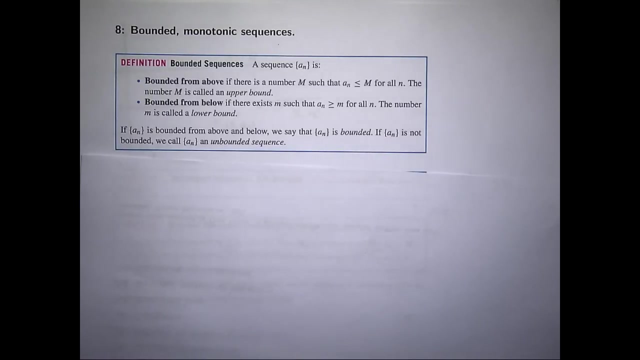 So this middle sequence is a bounded sequence because it's bounded above by some number and below by some number. This sequence also is bounded above and below. Okay, so there's some examples. There's some examples of some bounded sequences. Let's just, you know, think about some sequence say sine n. 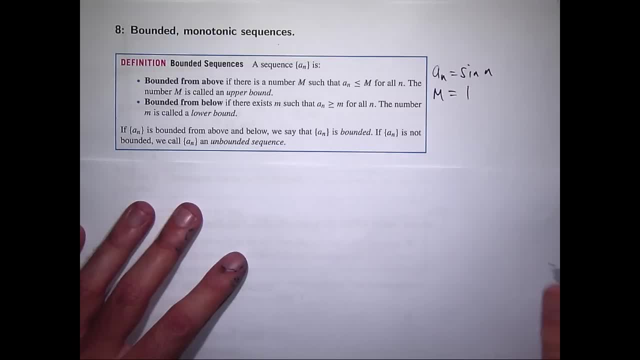 We know that sine's bounded here, so the upper bound would be positive 1, and the lower bound would be negative 1.. Okay, now, some sequences aren't bounded at all. They don't have an upper bound or a lower bound. 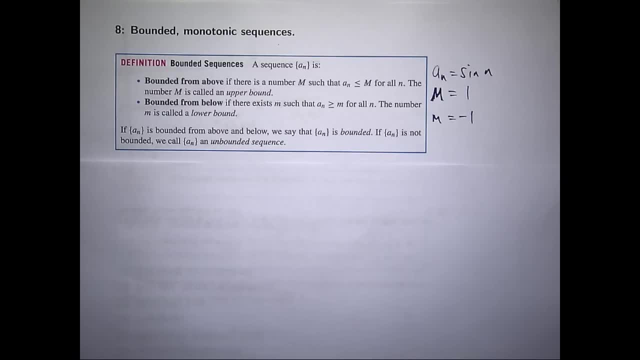 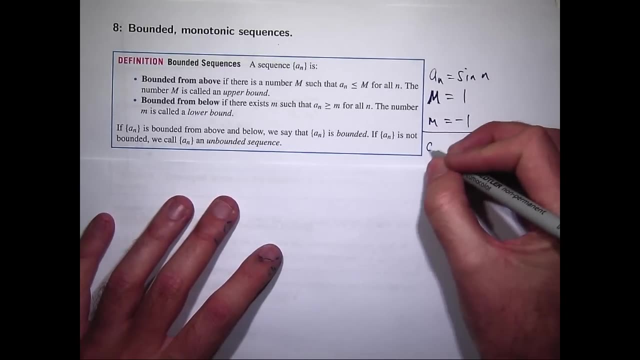 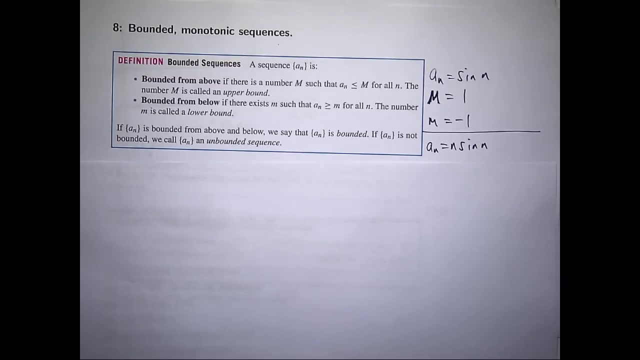 So, for something that's not bounded either above or below, think of something like this: Instead of sine n, what about n sine n? Okay, that sequence is neither bounded above nor below. Now these values, at least for this sine n. 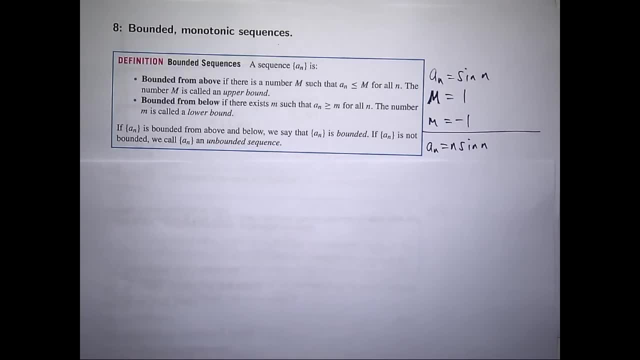 I've just chosen big M to be 1 and little m to be minus 1.. I could choose other values like big M equals 2, big M equals 100, little m equals minus pi. They're still correct. Okay, there's still bounds on the sequence. 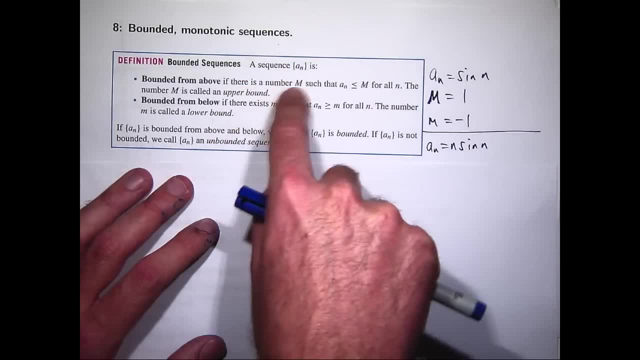 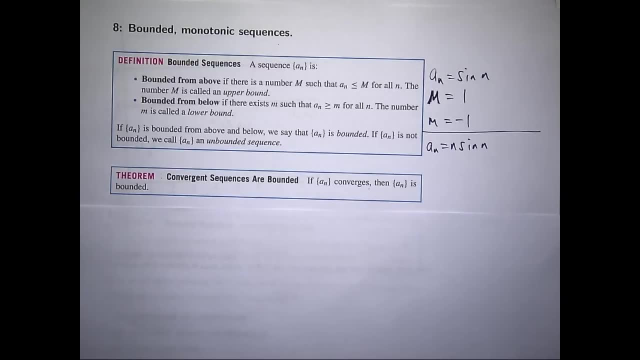 So there is a number, not necessarily a unique value. Okay, an important theorem: convergent sequences are bounded. That is, if we have a convergent sequence, then that sequence must be bounded, Okay. conversely, if you have an unbounded sequence, 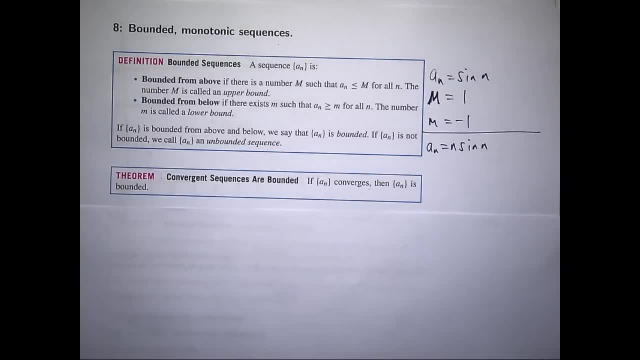 okay, from a practical point of view, if you have an unbounded, if you have an unbounded sequence, then it can't converge. Okay, That's probably of more practical use And this is the main theorem here. Okay, I think in your notes I've removed one picture. 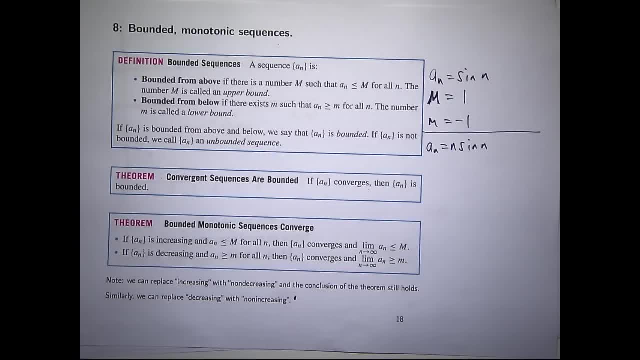 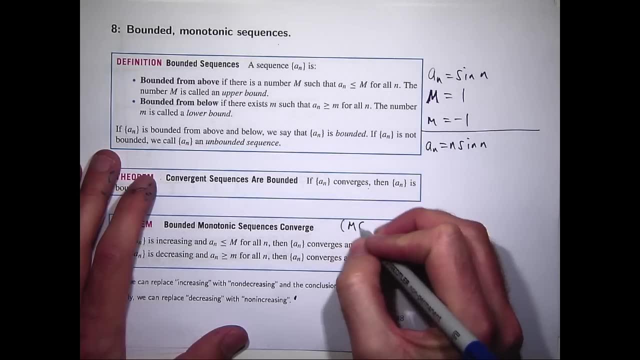 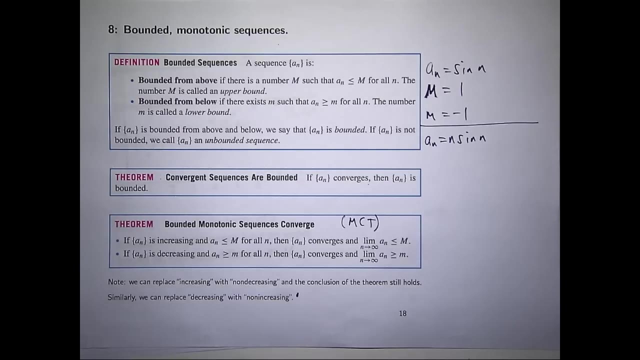 because I thought it was slightly unclear, but it should be okay. The monotone convergence theorem. Okay, The MCT. Now when I talk about an increasing or a decreasing sequence, it's kind of like an increasing or a decreasing function. 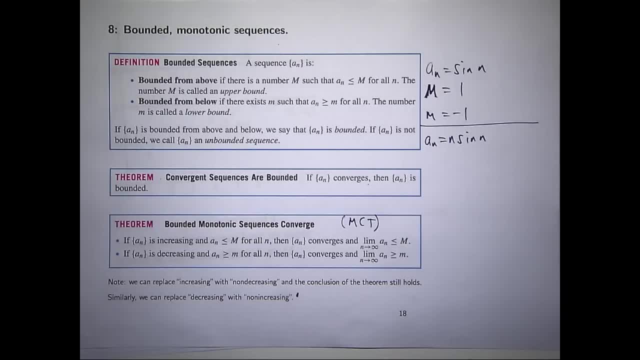 Okay, You can think of. you know you're either heading up as you move along the sequence, or heading down. So what does this monotone convergence theorem say? If we have an increasing sequence that's bounded above, then the sequence must converge. 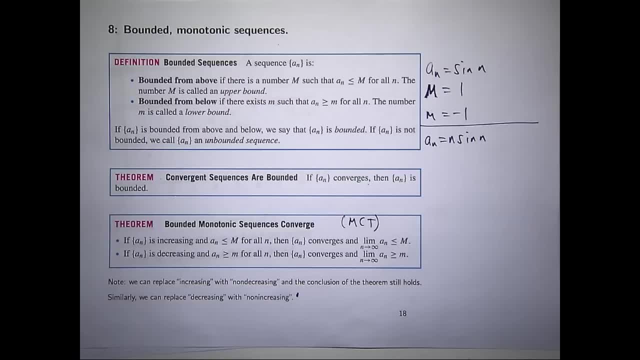 And secondly, if the sequence is decreasing. if a sequence is decreasing and bounded below, then the sequence converges. Okay, Now it doesn't these theorems. it's slightly abstract, the monotone convergence theorem, because it doesn't tell you what the limit is. 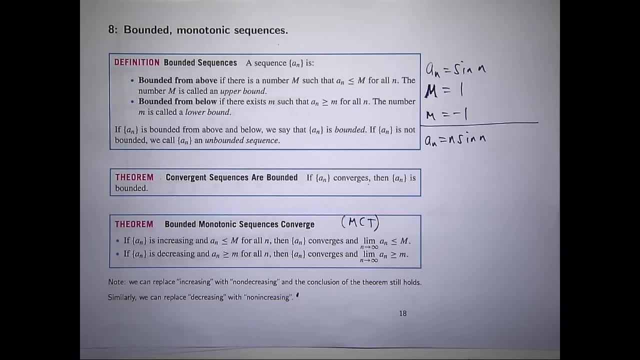 Okay, It just tells you that the limit exists And in the first case, the limit is less than or equal to this upper bound, And in the second case, the limit is greater than or equal to the lower bound or a lower bound. 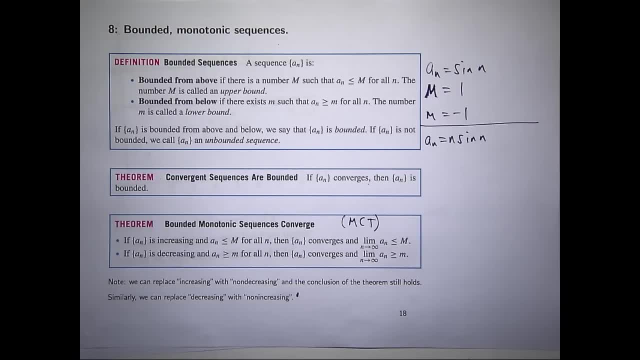 Okay, It's very powerful. It's something that you can use all the time just to show that a limit actually does exist. Okay, Now, I'm not going to prove it, but we are going to look at how we can apply it. 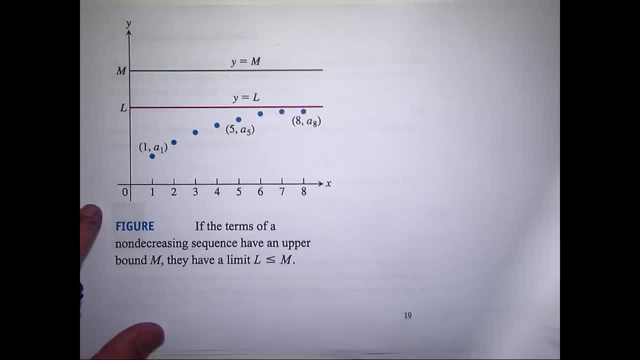 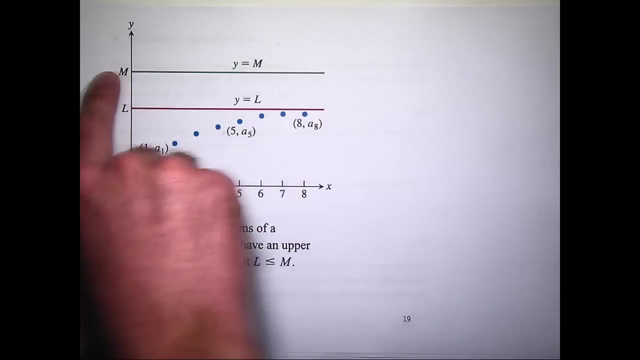 Okay, But before we do that let's have a look at geometrically what's going on. Suppose I've got a sequence Here. it's just plotted in the plane And M big M is any upper bound for the sequence, What you can see from the picture. 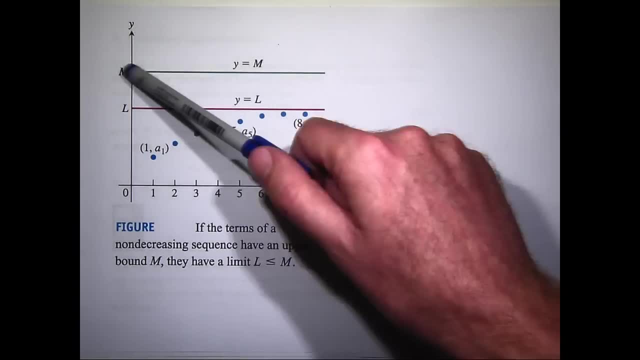 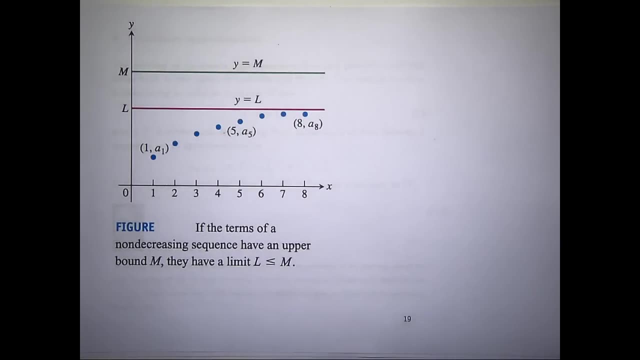 the sequence is increasing and it's bounded by this, this number, big M. What the monotone convergence theorem says is that the limit of that sequence does exist and the limit is less than or equal to whatever that number big M is. 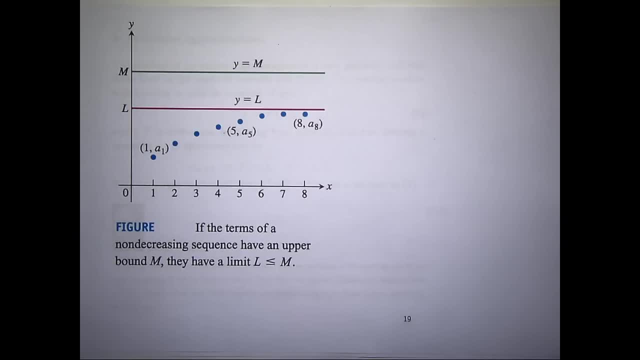 Okay, So you can see, in this case, the limit is actually less than big M. Okay, So it's like a graphical representation of what the monotone convergence theorem says. Okay, So it's a very powerful theorem and it's something that you'll use quite a lot. 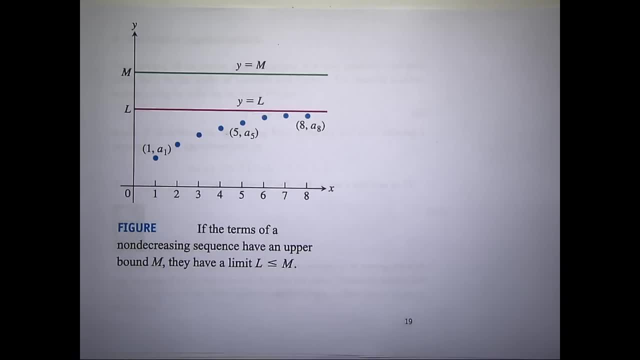 in this course. Now, it does have limitations. It's very general, but it does have limitations in the sense that it doesn't tell you, at least in the form that I presented, what the limit actually is. All you know that it's less than or equal to. 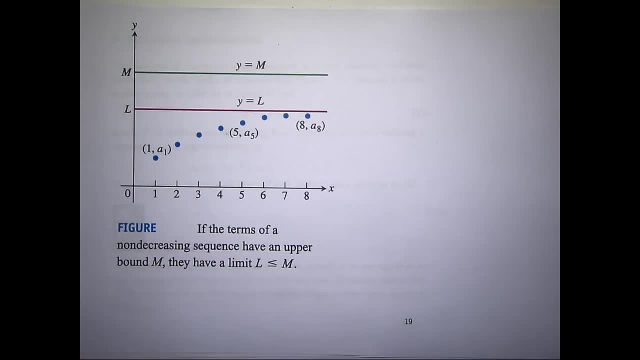 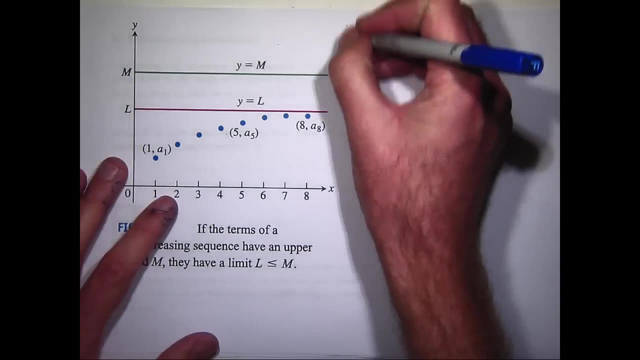 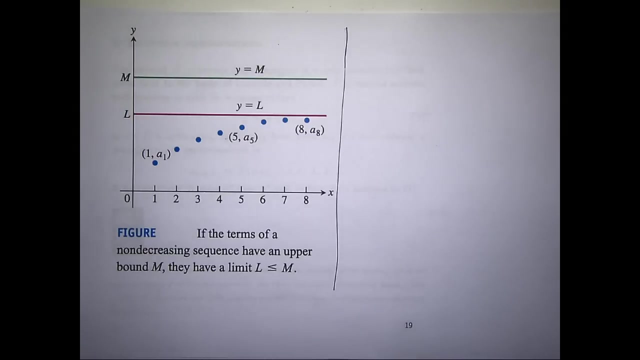 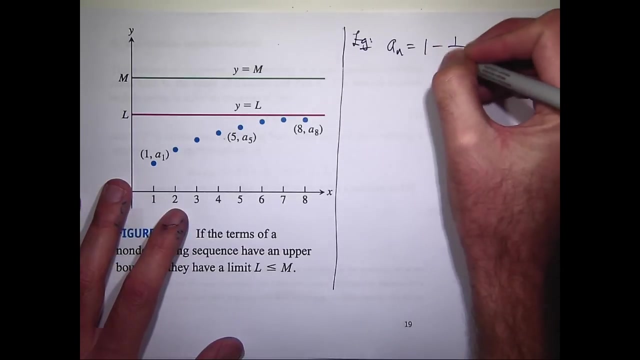 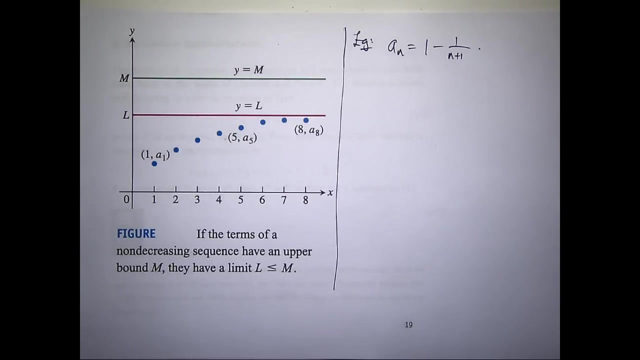 your bound on the sequence. Okay, Now let's have a look at an example. Say this sequence here. Now, this sequence is an increasing sequence. Okay, Now you can also easily bound this. let's say: you know, 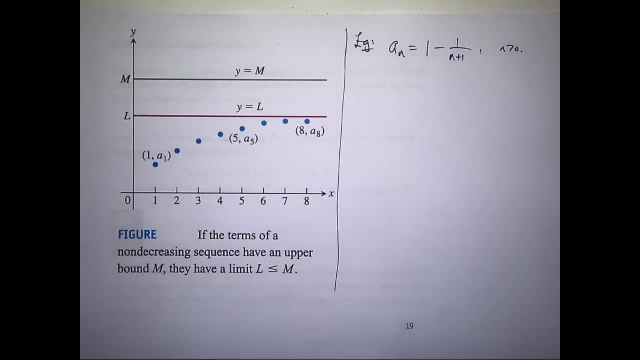 it's N greater than zero. You can easily find an upper bound for this particular sequence. Anyone. One One's a good choice, But you can also have an upper bound of two, Three, A hundred Sixty-four, Okay. 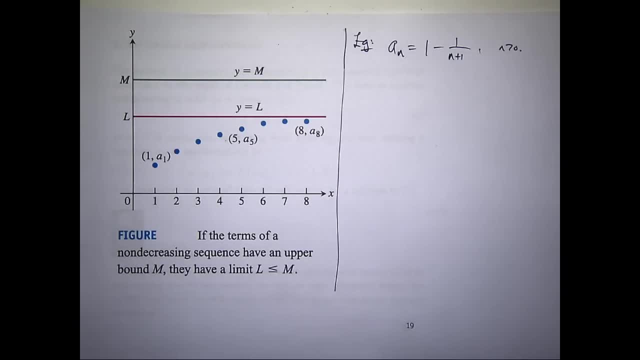 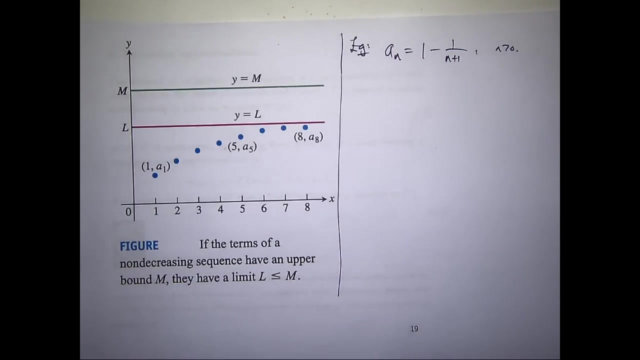 They're all correct. They are all bounds, upper bounds for that sequence. But think of all the upper bounds for this sequence. What's the smallest one? Positive one? Okay, Now this converges to one in the limit, right? 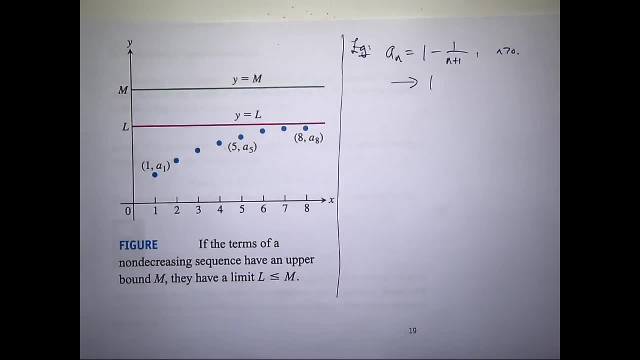 Let's just go to zero. Now this, the, the one, is a special bound. Of all the upper bounds, one is the least, the lowest upper bound. Okay, So, although I haven't explicitly stated it, the monotone convergence theorem. 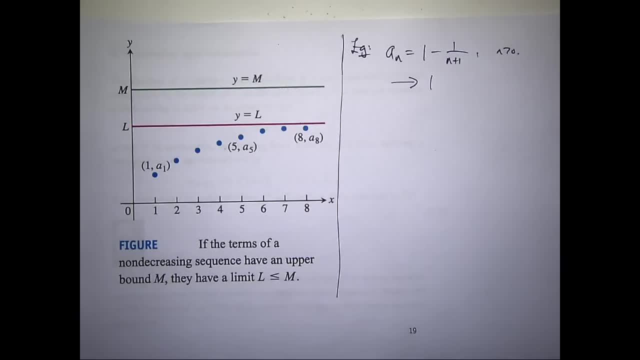 does give you a little bit of constructive information. If you have, say, an increasing sequence that's bounded above the limit does exist and the limit so-called least upper bound, Okay, So of all the all the upper bounds, 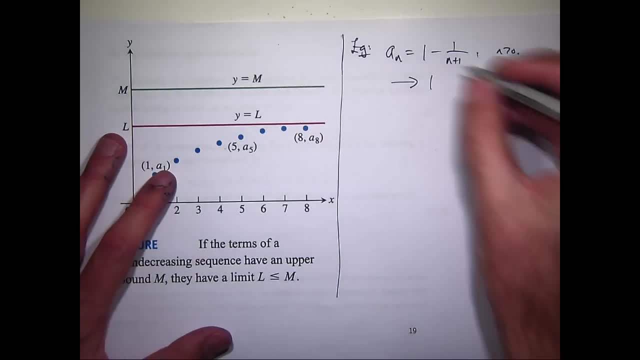 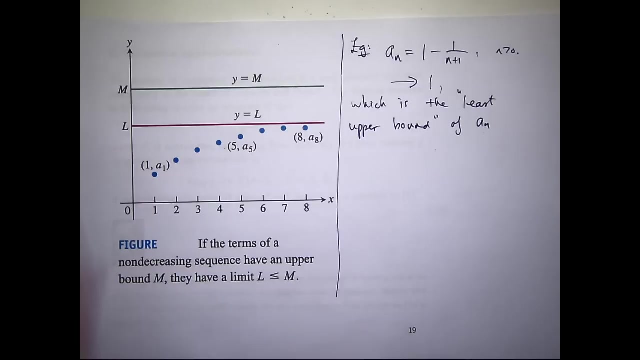 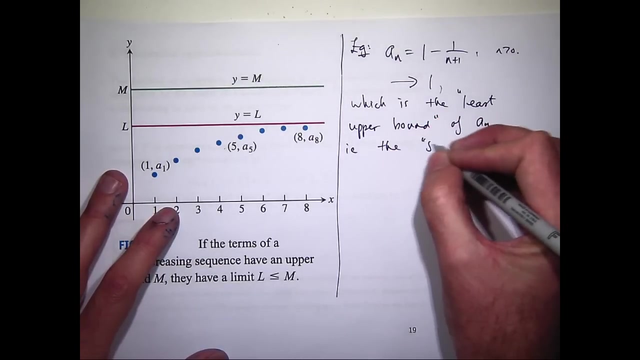 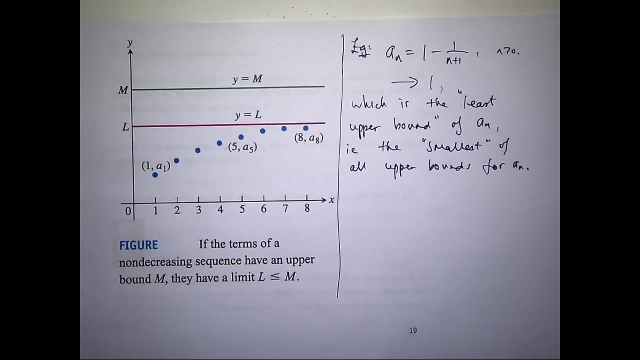 it will converge to the least upper bound. Okay, Okay. So to put this into some sort of practical context, let's go back to the. I'll put this up in a minute. let's go back to this picture. Let's think about one on n. 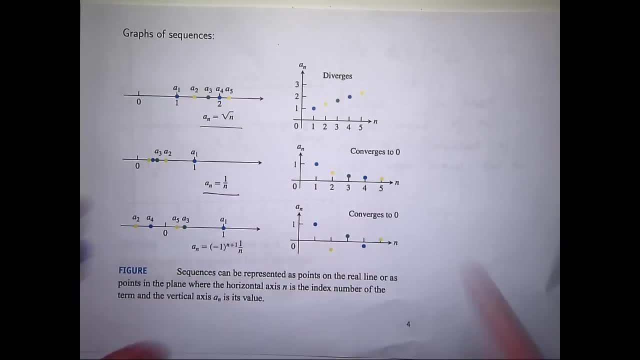 okay, the sequence one on n. That is a decreasing sequence that is bounded below by lots of numbers: minus 100, minus 10, minus 5, minus 4, minus 3,, all the way up to zero. Zero is the. 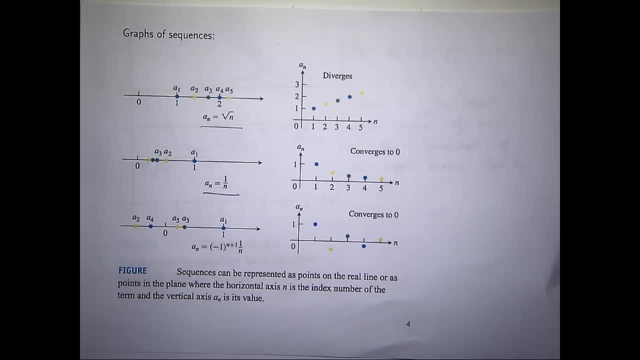 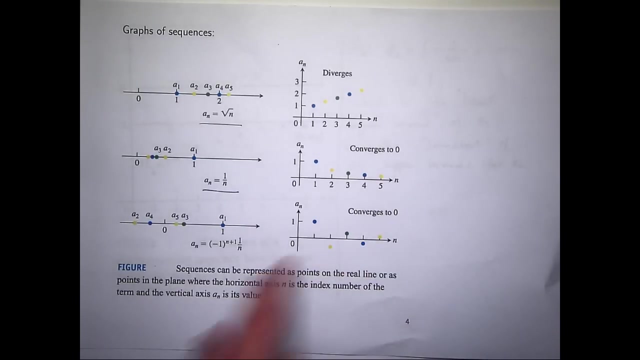 greatest of all the lower bounds. You can see that, of course, one on n converges to zero. It converges to its greatest lowest lower bound. okay, Now, this sequence here is neither increasing nor decreasing. okay, So you can see that it doesn't converge. 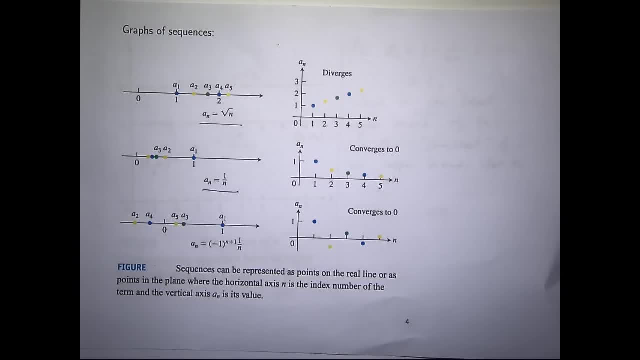 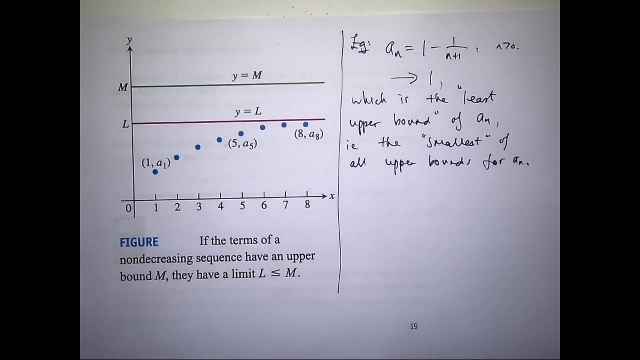 to either its greatest lower bound or its least upper bound. It converges to something in the middle right. So the monotone convergence theorem is really tied with bounded and monotonic sequences. Okay, so this is. yeah, this is important. 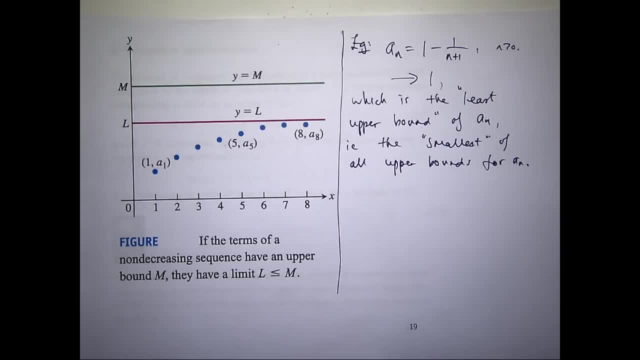 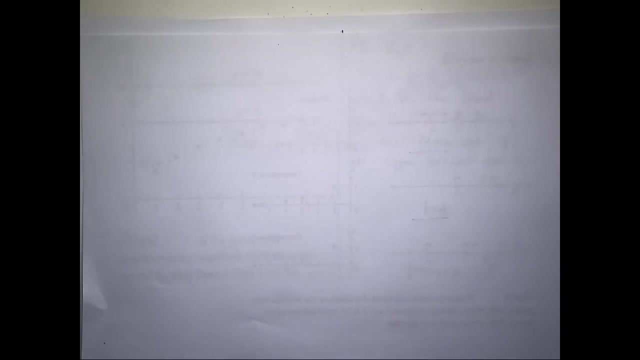 This is something that you can use. Let me show you another application of the monotone convergence theorem. So I don't have this written down, but this is actually one of your tutorial problems. Okay, so you might just if you've got a bit of extra space down here. 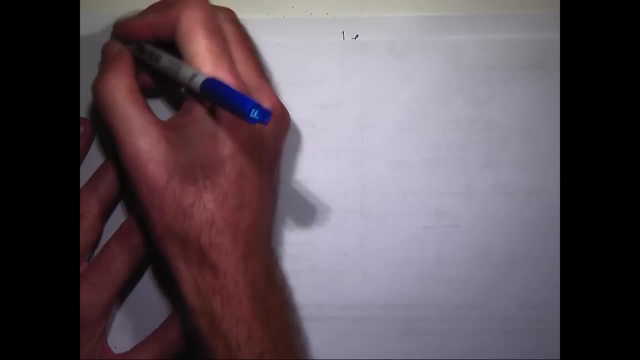 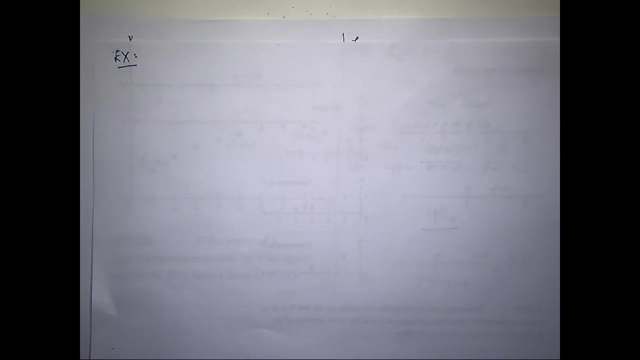 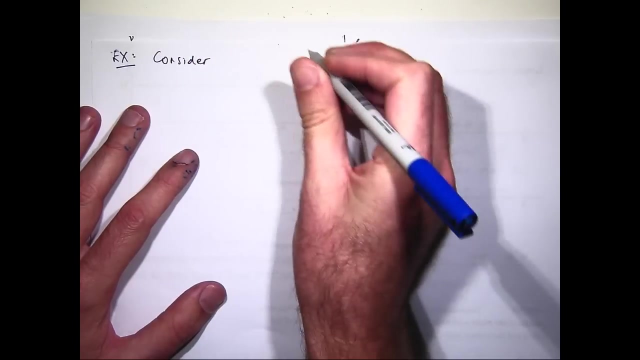 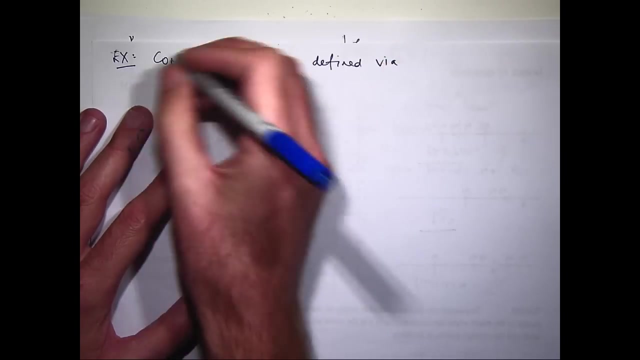 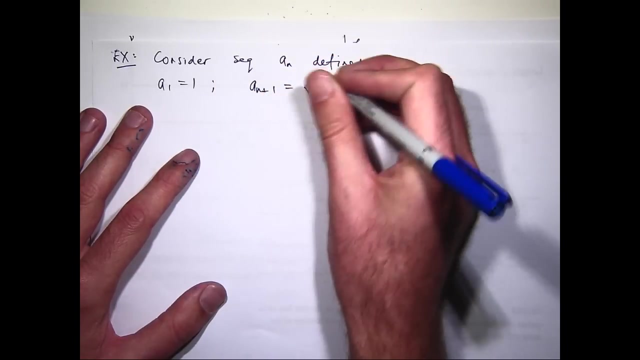 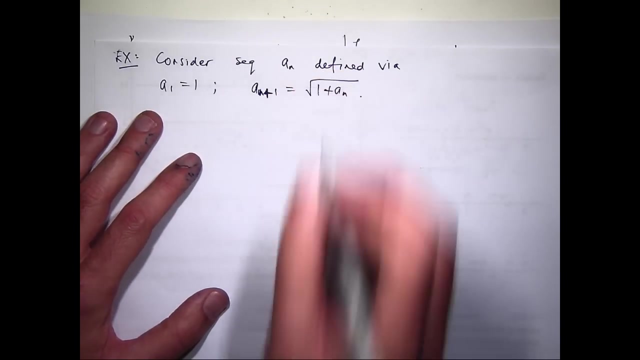 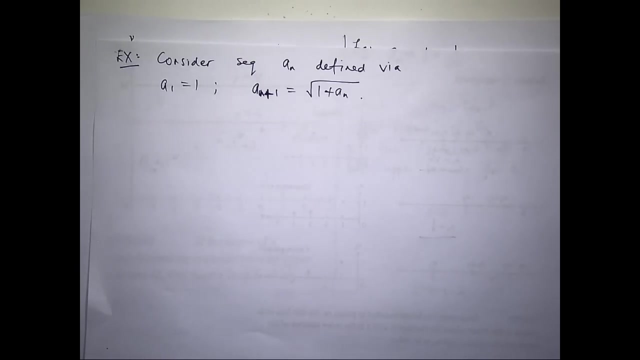 you might wanna sort of see if you can fit it in here Now. I can define a sequence in the following way: a so-called recursion relation, Yeah, Okay. so this is kind of like a what we refer to as a recursively defined sequence. 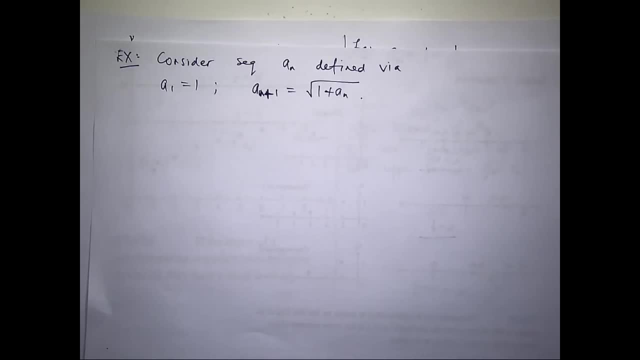 You start with some value of the sequence, a sub one- in this case it's one- and then to generate a sub two, you use this over here, So you put one into here and a sub two would be root two. 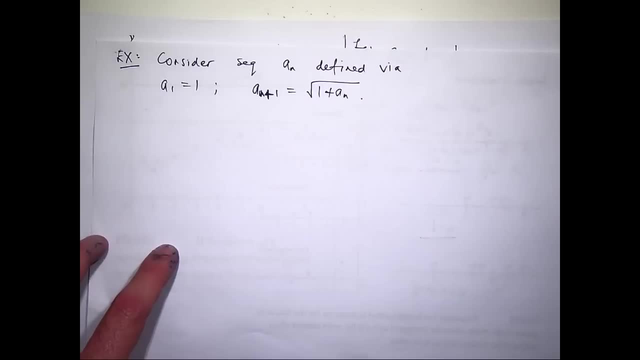 Okay, then, to get a sub three, you would put a sub two back into here and work that out. Now this particular question asks you to show that the limit exists and calculate the limit of a sub n. Okay, So that's what we're gonna do. 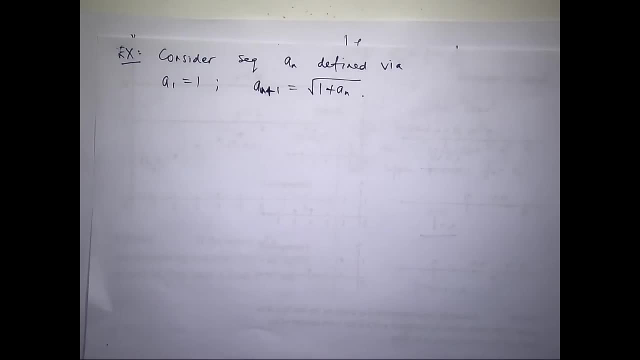 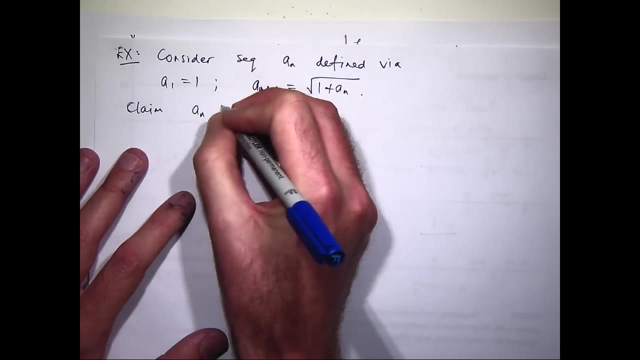 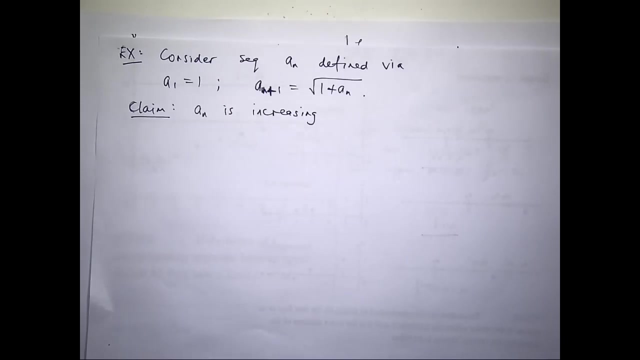 We're gonna use the monotone convergence theorem to do it. Okay, so, Essentially, all we need to do is tick off the two conditions of the monotone convergence theorem. We want to show that the sequence is monotonic: it's either increasing or decreasing. 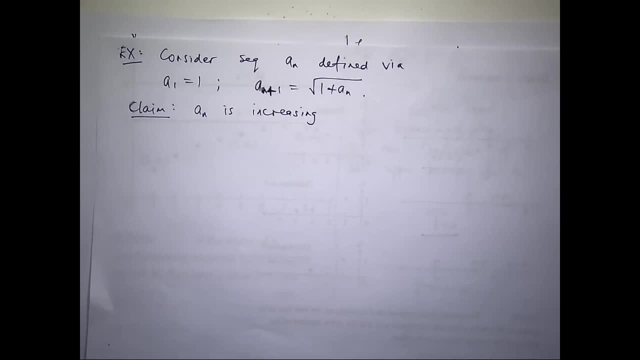 and it's bounded either above or below, depending on what you know, whether it's increasing or decreasing. If we can tick off those two claims, then we know the limit must exist, And then after that it gives us a little bit of a hunting license. 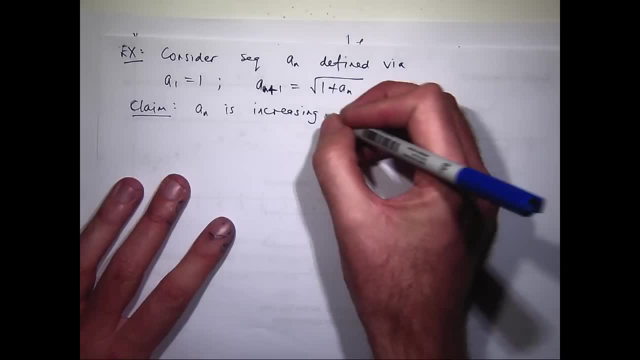 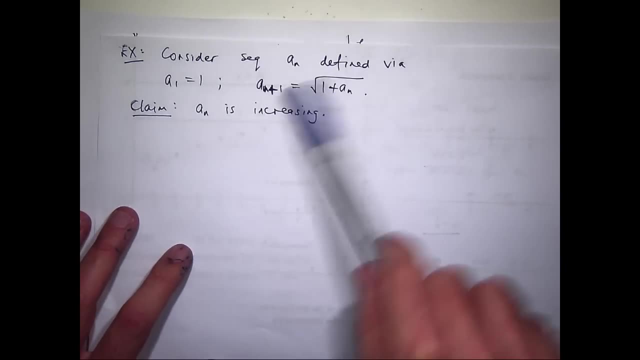 Maybe we can go and hunt for the limit, Okay, Okay. so how do we do this? Well, sometimes you can play with this and look at the ratio of a sub n plus one over a sub n and show that's either strictly greater than one or strictly less than one. 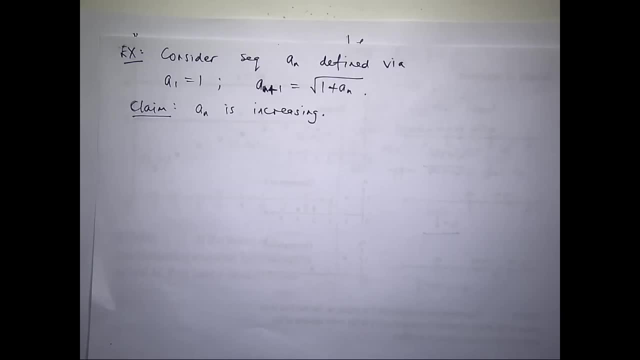 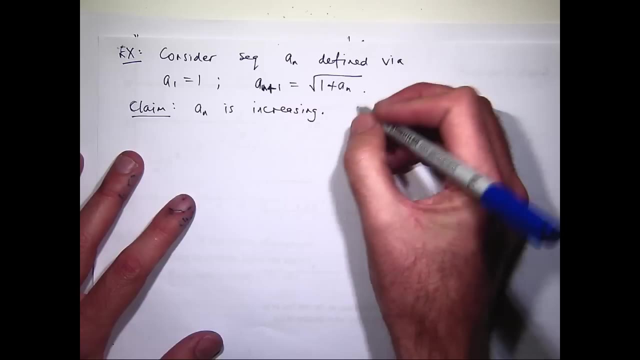 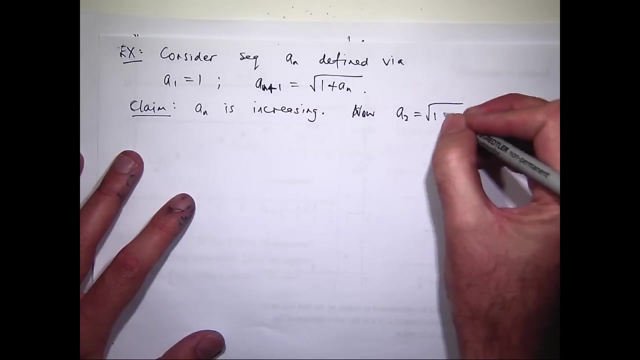 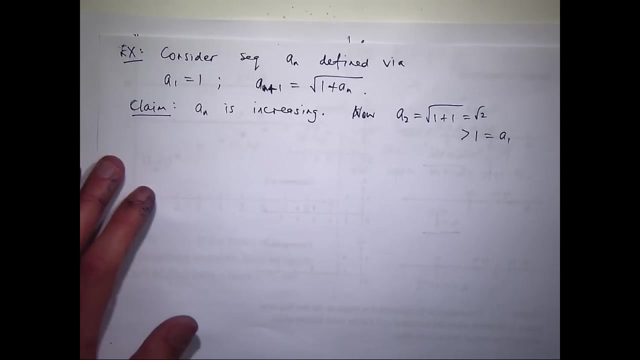 But this one isn't so easy, so what we're gonna do is use induction. Okay, So let's have a look. A sub two, that is root one, plus one root two. okay, Root two is greater than one, which is a sub one. 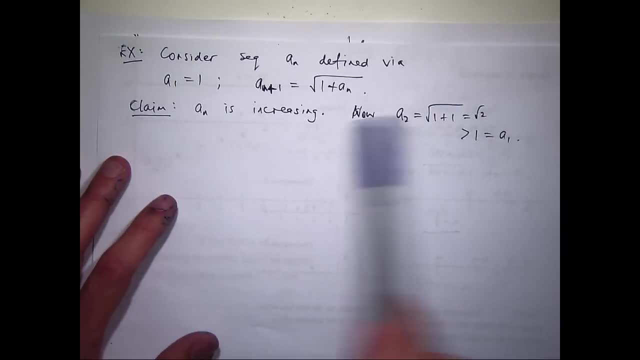 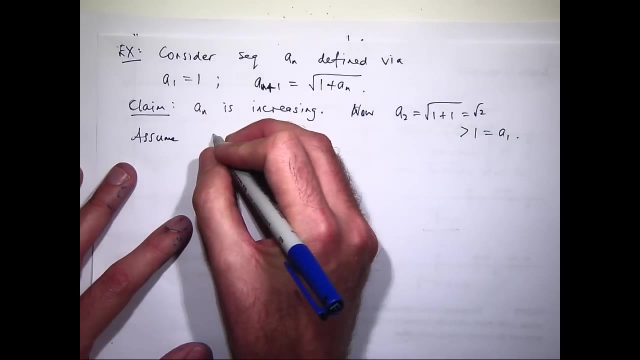 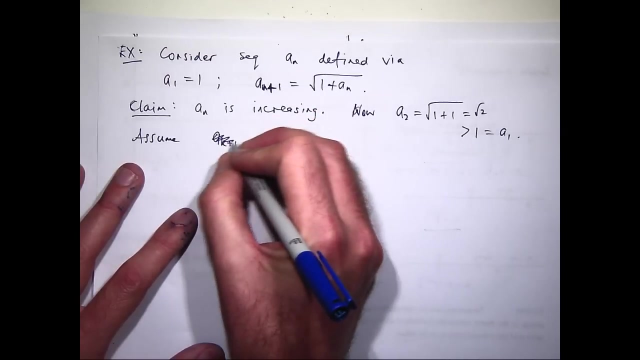 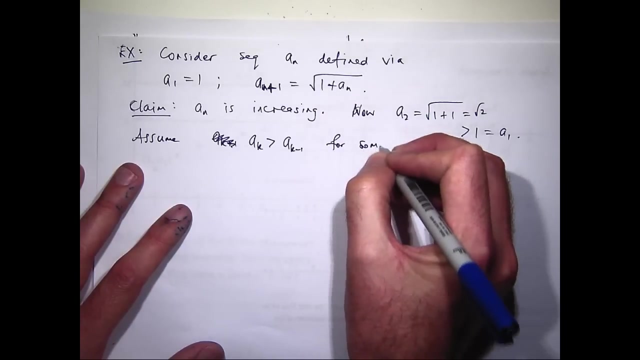 so it's true for this first case. So we assume A sub k plus one actually, let's, let's use that A sub k is greater than a sub k minus one, Okay, So what we would like to do, then, is show that this is true. 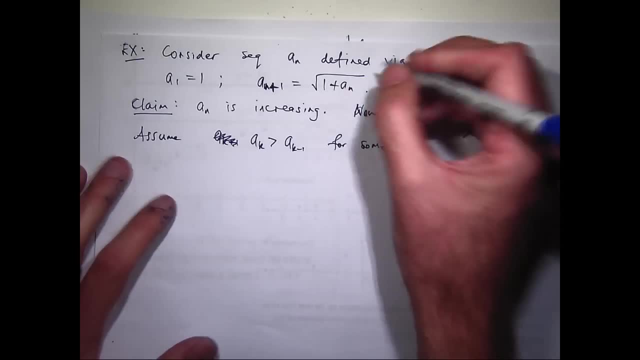 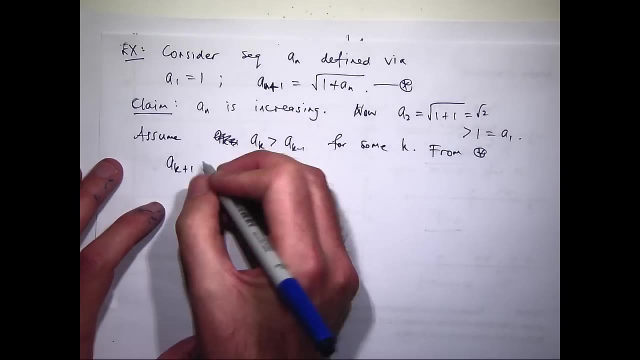 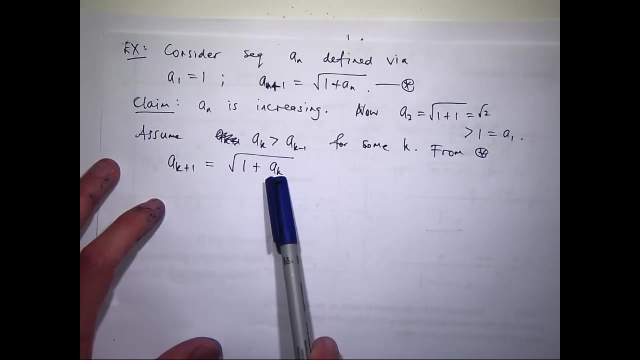 A sub k plus one is greater than a sub k. So let's see, A sub k plus one is greater than a sub k. Okay, So let's see. So let's consider this Now. A sub k is by assumption. 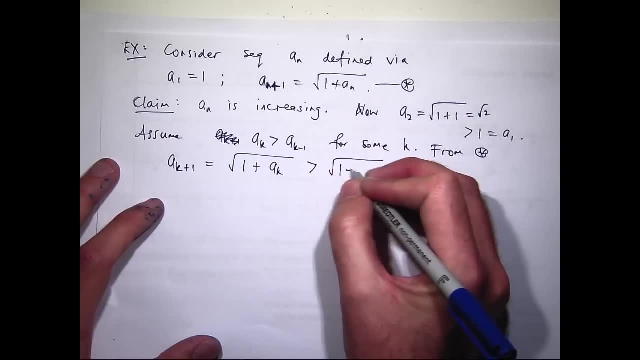 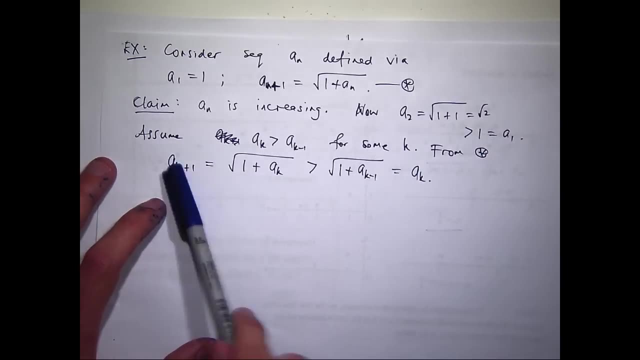 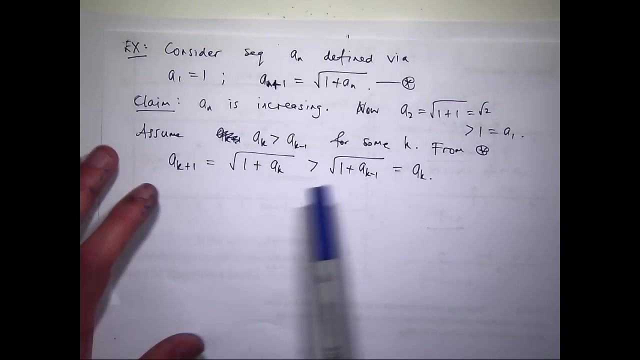 is greater than a sub k minus one. And what is this? Well, that's just by definition a sub k. So I've got my inequality: A sub k plus one is strictly greater than a sub k. So by induction, then this must be true for every n. 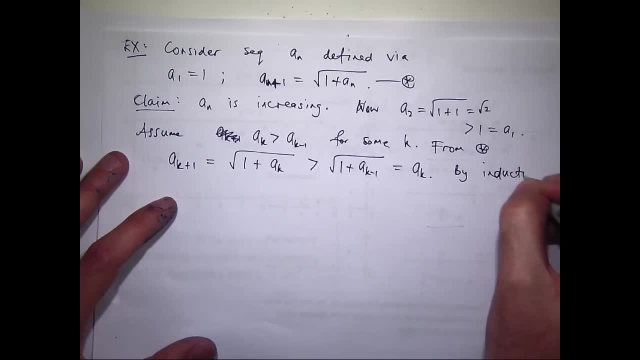 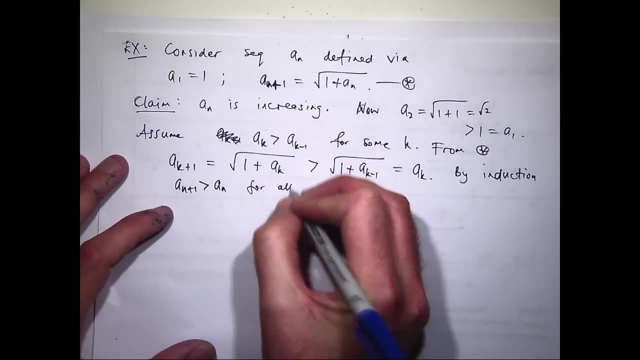 but, by the way, a sub k plus one is simply greater than a sub k. So I ran my homologous equation, which I can call it the noise equation. But then let's say I'm going to do the same thing. 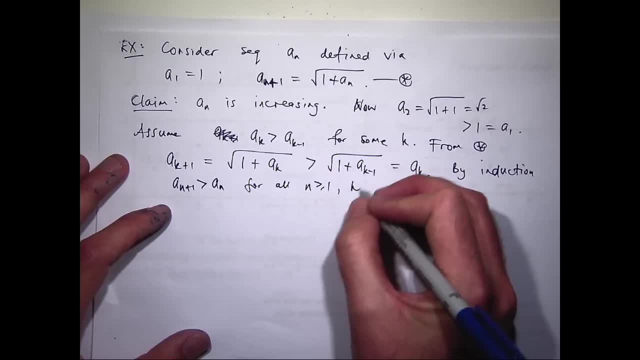 with all these n's. I'm going to do the same thing with my homologous equation. So A sub k plus one is a sub k minus one. I'm going to do the same thing with my homologous equation. So here's my monotonic. 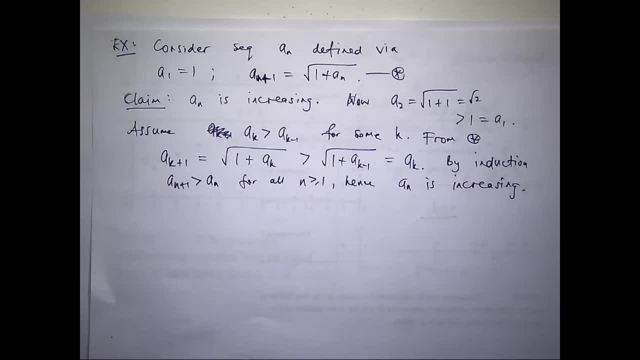 Let's say, I'm going to do the same thing with a sub k. So let's see, I've got the gårer, so I'm going to do the same thing with the sub k. What's the solute here? OK, Okay, So that's one half of the conditions. 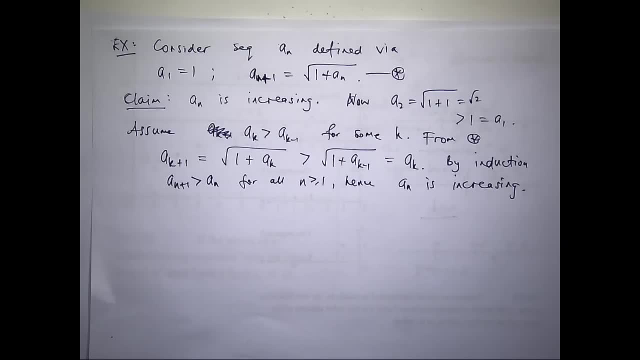 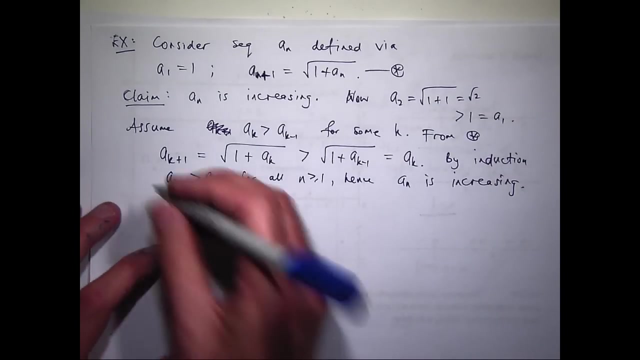 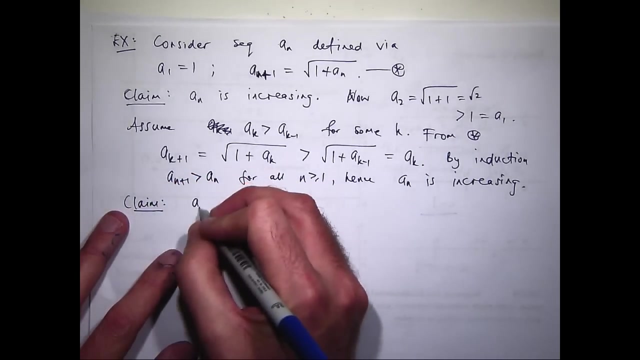 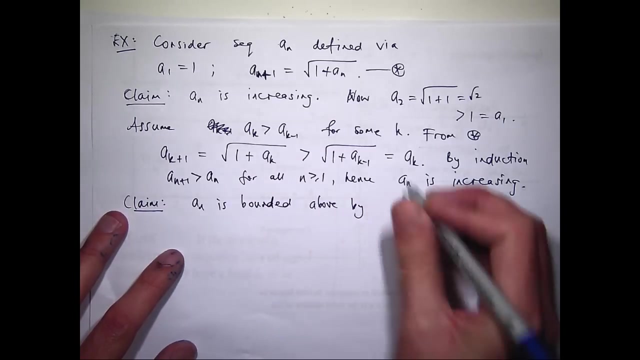 monotonic. Now if it's increasing, what I would like to do is show there's an upper bound for every a sub n. Now it can be tricky choosing the upper bound here, and sometimes you have a bit of a hint. I'm going to make the following claim: a sub n is bound to the. 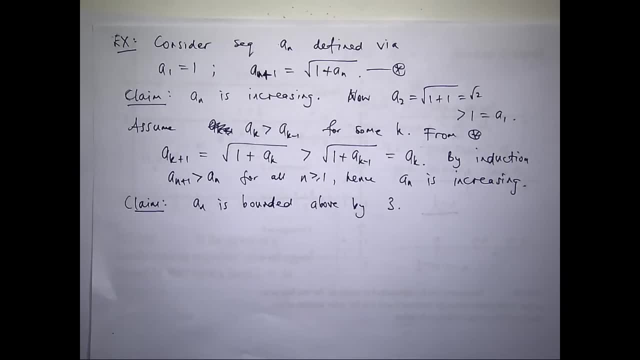 bulk by positive 3.. Now, you don't need to have positive 3 here, Just positive 3 works well. okay, You'll see why in a minute. Okay, you could have any sufficiently large number there. Okay, so again, let's do it. 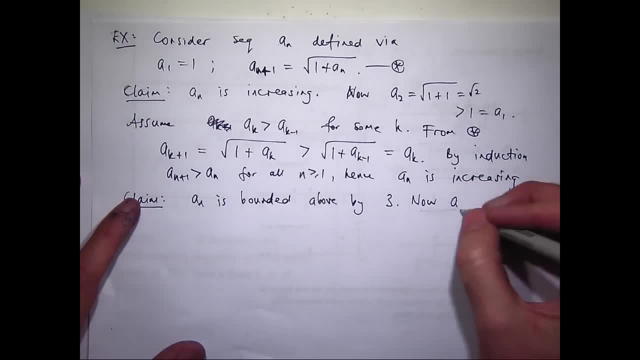 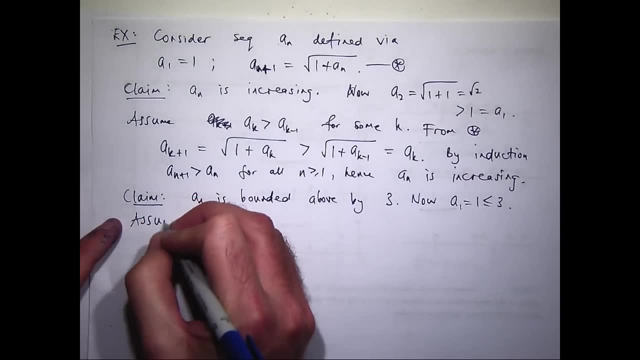 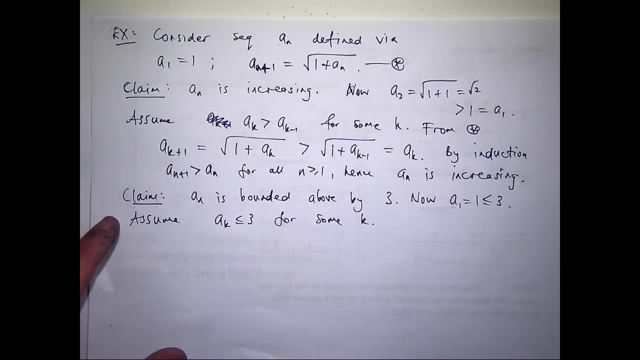 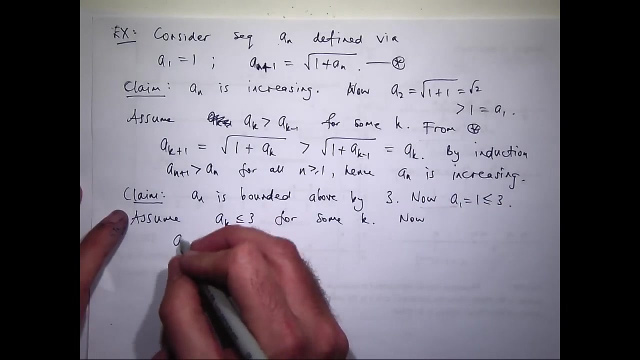 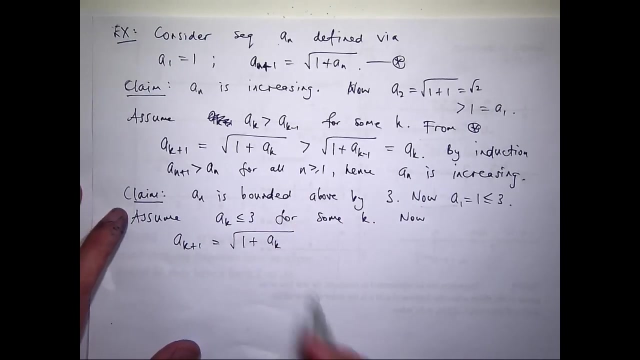 by induction. a sub 1 is 1.. That's certainly less than or equal to 3,, isn't it? Yes? So let's assume it's true for some k strictly greater than 1.. a sub k plus 1.. Well, by definition, it's just that, with n replaced by k And by our 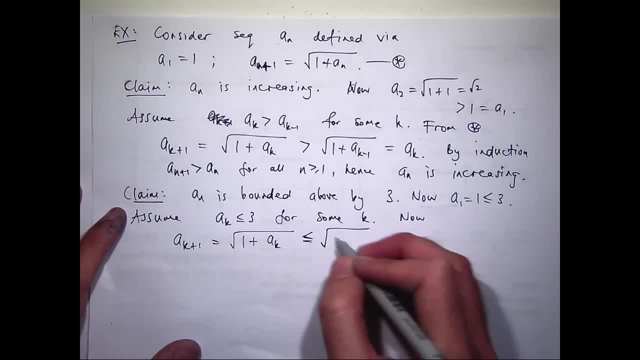 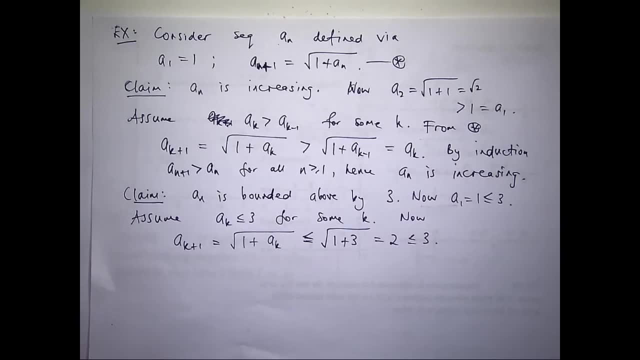 assumption: a sub k is less than or equal to 3.. So it would be less than or equal to root 4,, which is just 2.. Now is that less than or equal to 3?? Yes, it is Nice Okay. 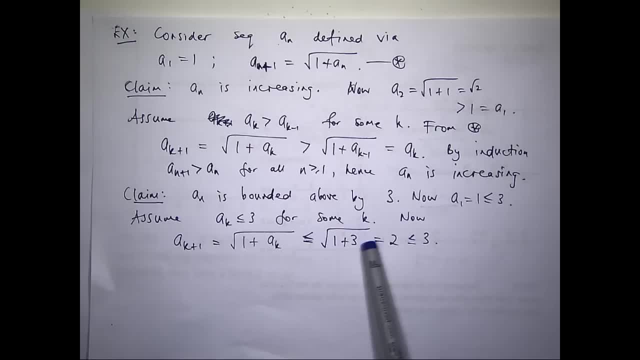 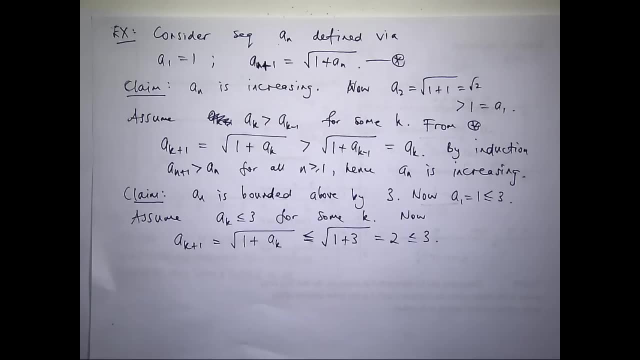 you can see how the choice of 3 there was quite Okay If you wanted to work out. simply, a good choice is kind of required there. So what does it mean? Well, it means by induction, a sub n is bounded above by 3.. So, okay, our. 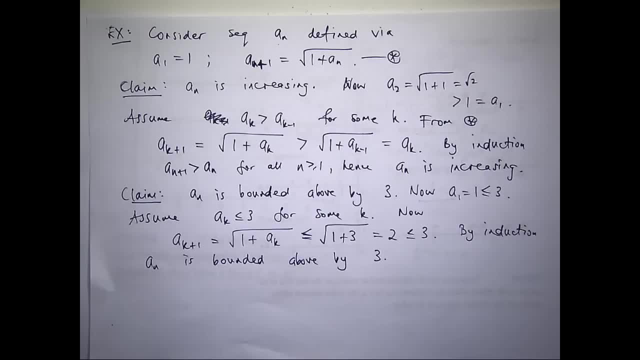 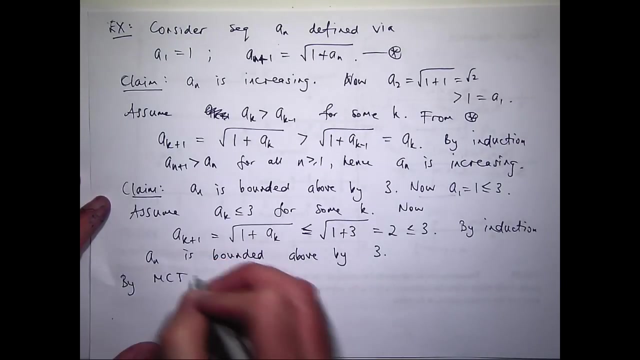 two conditions of our monotonic convergence theorem are now satisfied. We definitely know the sequence recursively defined by star is increasing and it's definitely bounded above by positive 3.. So what does it mean? It means that the sequence defined through star must have a limit. So by the monotone convergence theorem there is a number of 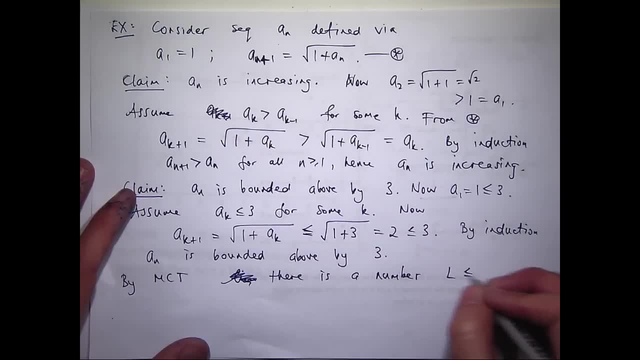 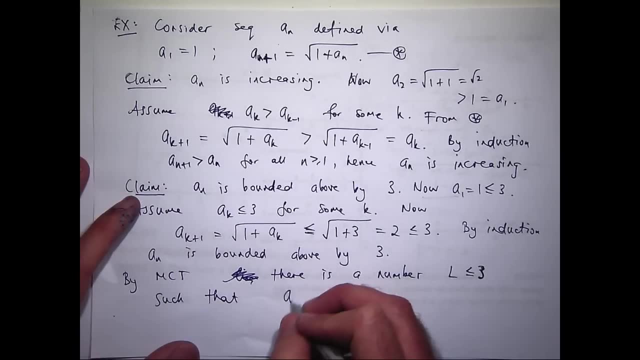 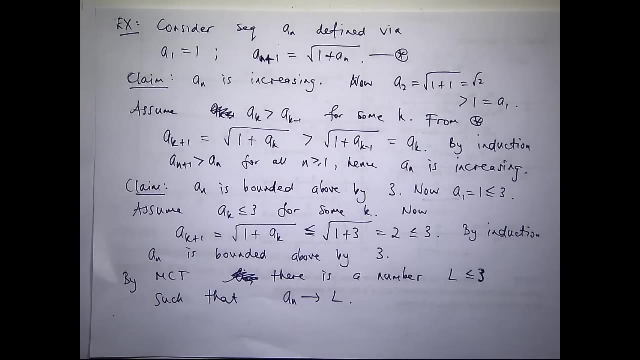 terms that we've already developed, or an order of turn. So we've got, you know, an average, a sub n which is less than or equal to 3, and n is less than or equal to 3,, so that, for instance, there's a constant l and n is less than or equal to 3.. And so 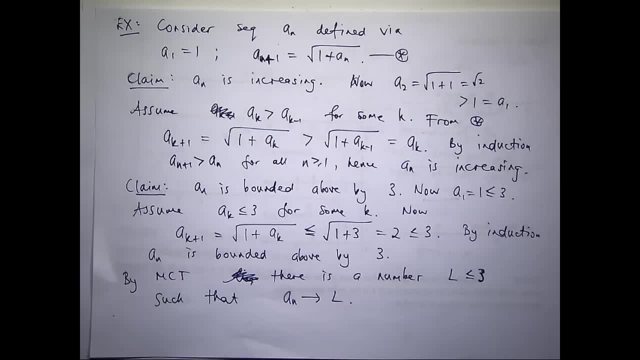 here we've got n plus l, Okay, And then then we put, let's say, l which is less than or equal to 3, such that a sub n converges to l. Now the next question, of course, is: well, how do I calculate l? What is the limit? 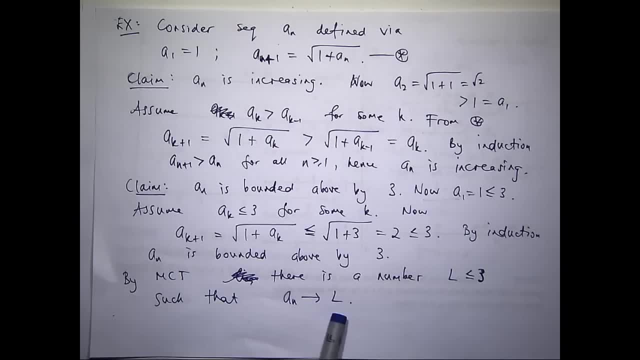 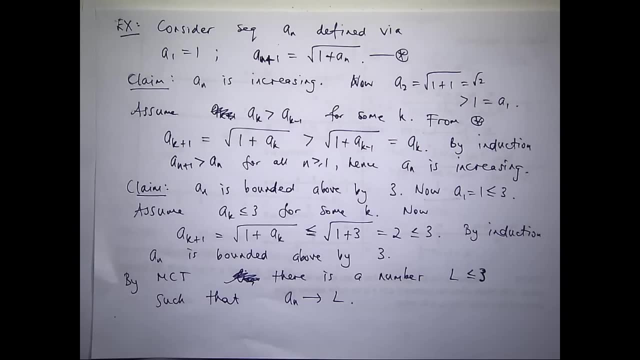 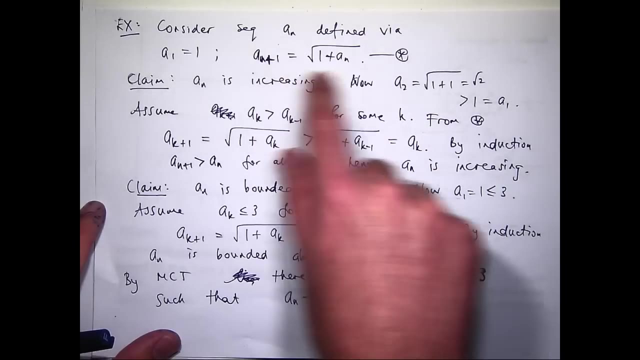 And some of you may already know how to do this. Any ideas, Any ideas? How might I calculate the, the limit? okay, i know it's less than or equal to three, but anyone, anyone, any ideas, any ideas? guess, well, essentially it's it comes from here. okay, having the subscript n plus one doesn't really. 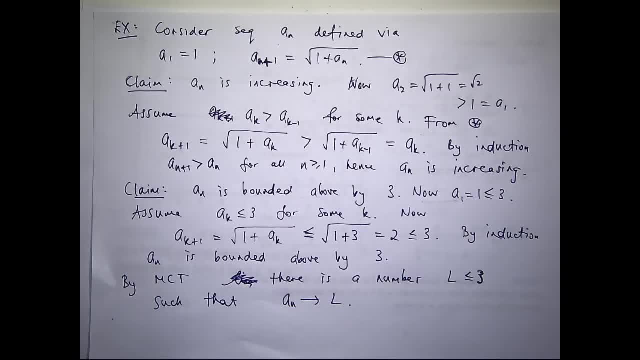 change anything, right? if a sequence has a limit. a sequence can only have if the limit exists. right, it's unique. you know, a convergent sequence only has one limit. so what does it mean? well, if i take the limit over here, i'll get l, and if i take the limit over here, i'll get root. 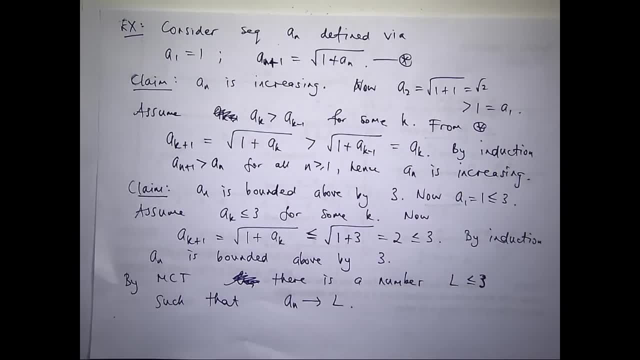 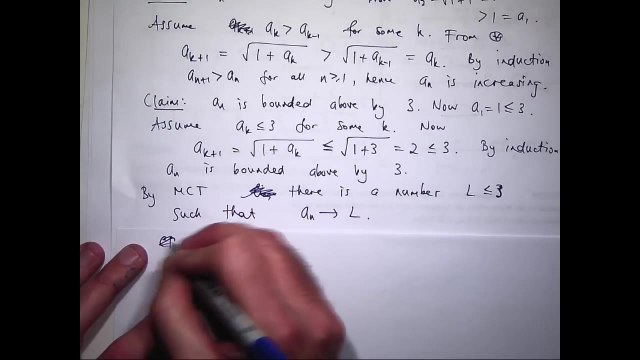 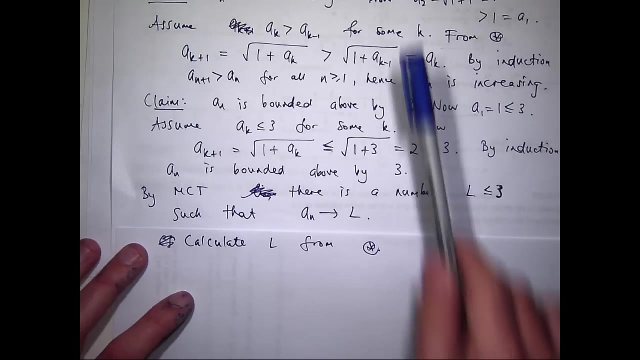 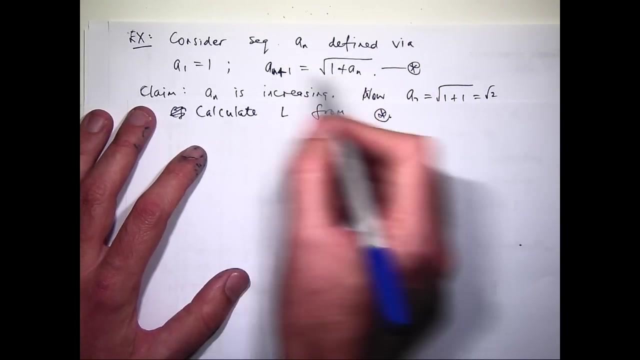 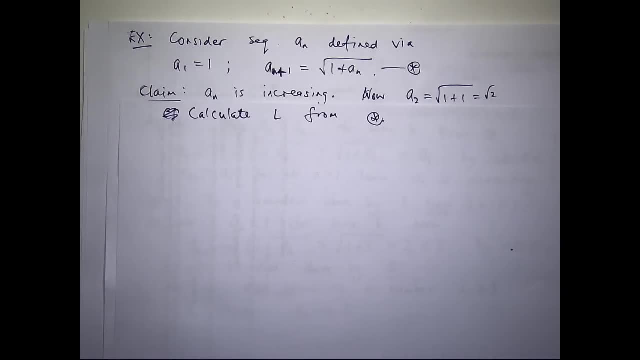 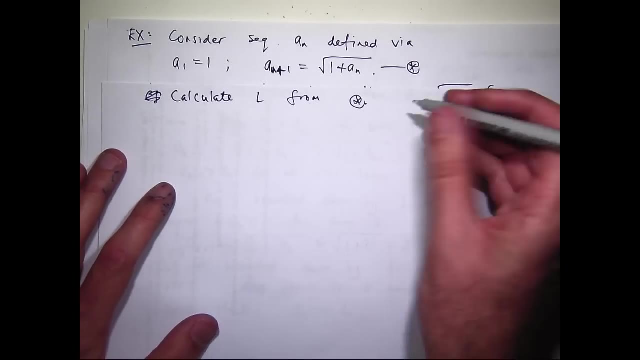 and i'll end up with l equals root, one plus l. now, that's not quite so easy to work with. so what i'm, what i'm going to do, is i'm going to take the limit over here and i'm going to get the other value i'm going to put in the left분. 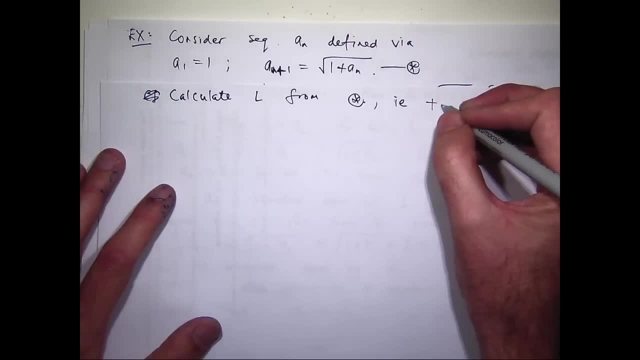 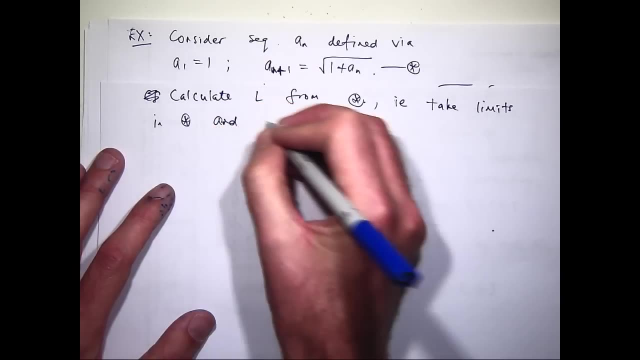 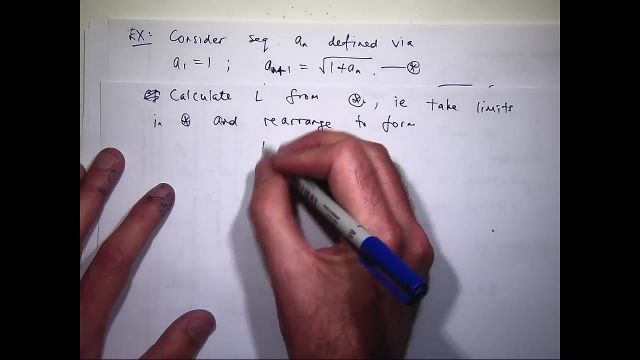 and two and two and three. there you go, okay, and after i do this, i'm going to- i'm going to get this equal to, okay, i'm going to get the element hero and i'm going to get a num smaller than that. that will be l, that will be l. i'll. actually, when i rearrange it, i'll get that. what is then? okay, so right. so i'll say l e k on la l gotten. and then right, Jack, it's gonna be four differently, not an object flat, but we're going to содерж it, but I'll get that, of course. 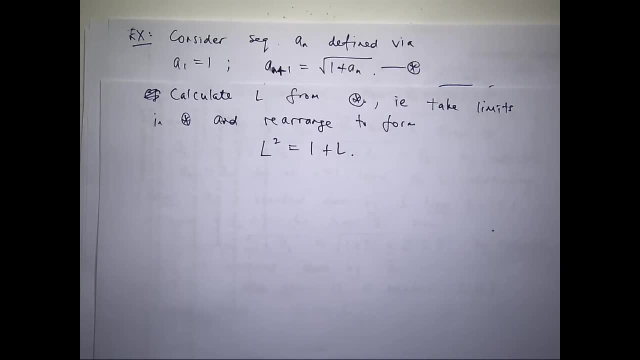 Now you may be a little bit worried here, because by squaring it I've actually introduced two values of L there. Yeah, So as long as we're careful when we solve this quadratic equation, you know we're going to get two values of L there. 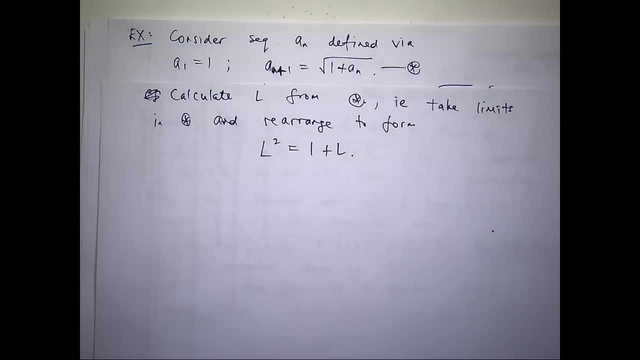 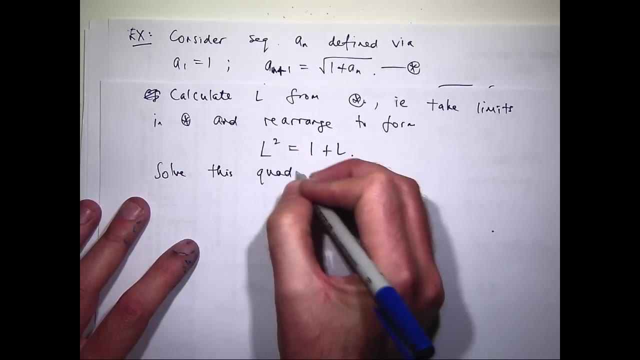 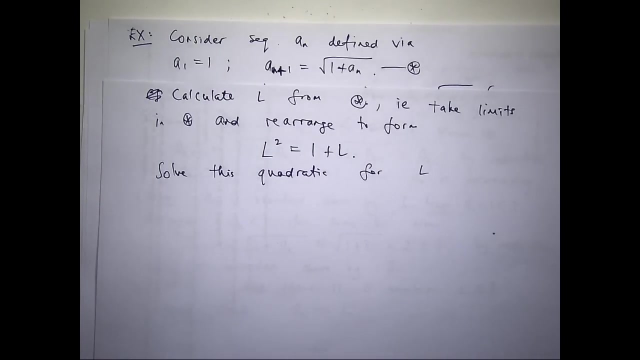 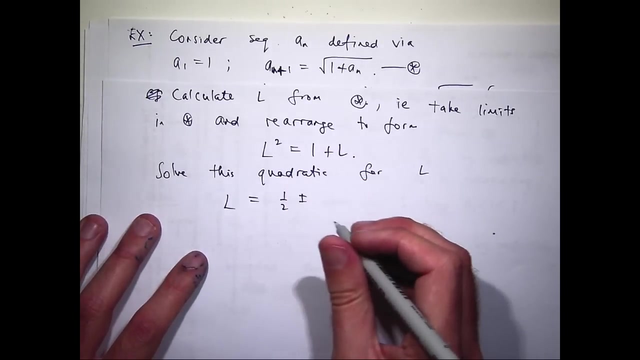 but we only want to select the one that we really want. Okay, Okay, so you can solve that in a variety of ways. I think I just completed the square and you'll get something like this: Is that right, Root 5.. 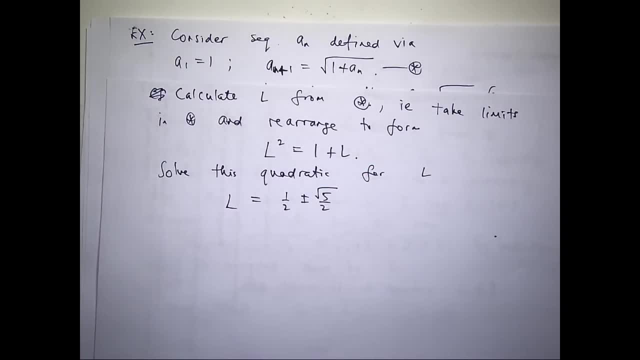 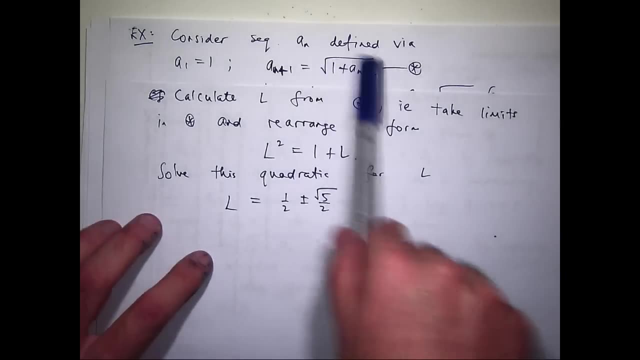 Root 5.. Okay, so Which one do we want? One of these is going to be positive, one of these is going to be negative. Well, we want the positive value for L because obviously the values of our sequence have got to be positive. 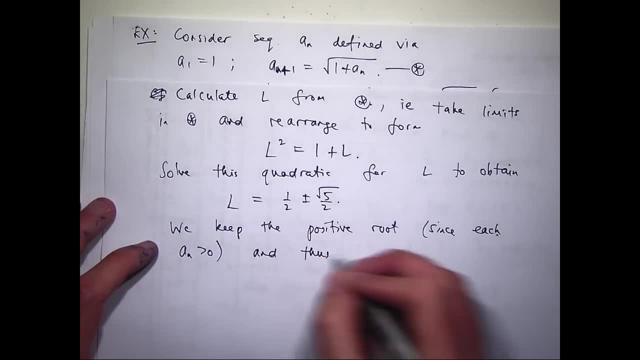 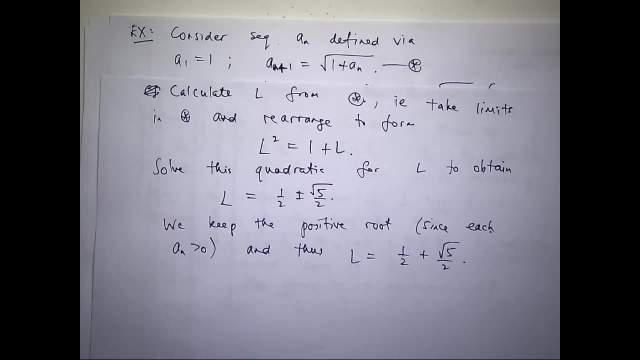 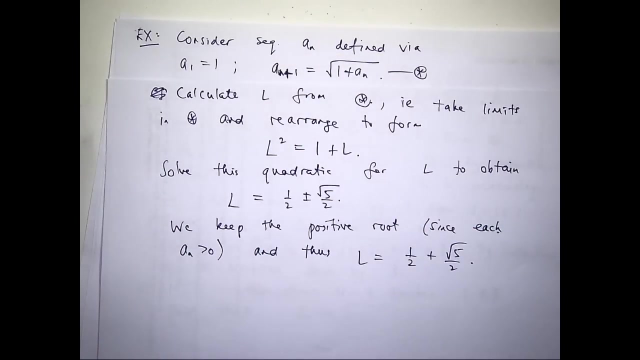 So the limit will be this. Okay, now some of you may be looking at this and going: hang on, Chris, why didn't I just start there, assume the limit exists and then go to that thing straight away? 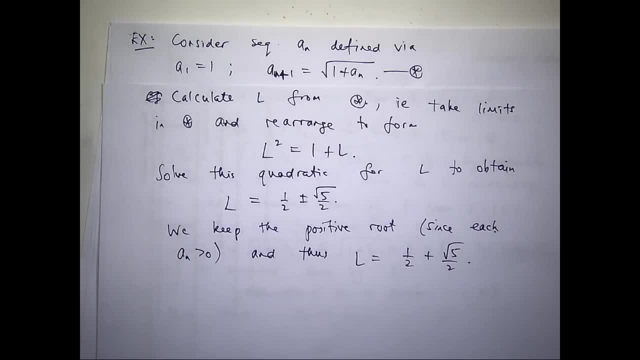 Well, you could do that. It's dangerous, though, if you don't know whether the limit exists or not. Okay, You don't know whether the limit exists or not, So you know, you're sort of scratching around there. 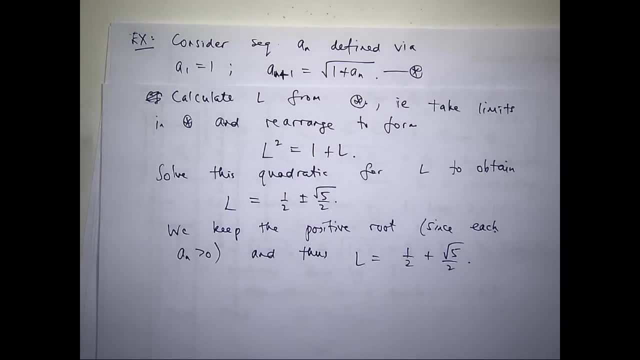 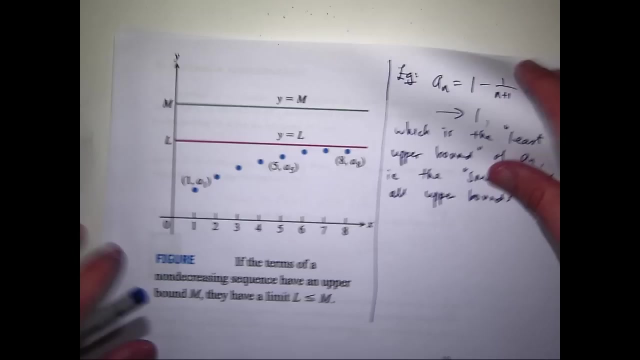 hoping something happens. That's a good, good question. Okay, one of your tutorial problems. So that's one sort of pseudo-application, but the following is slightly more definite. It's known as the method of success of approximations. 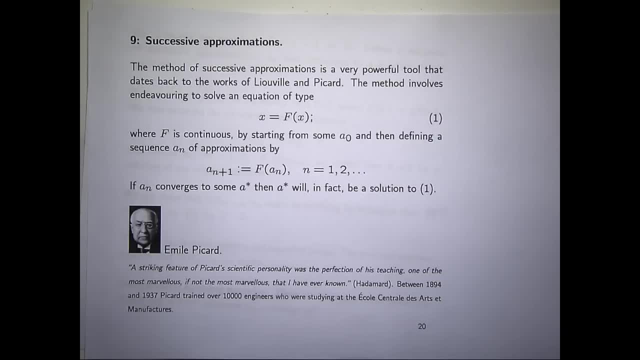 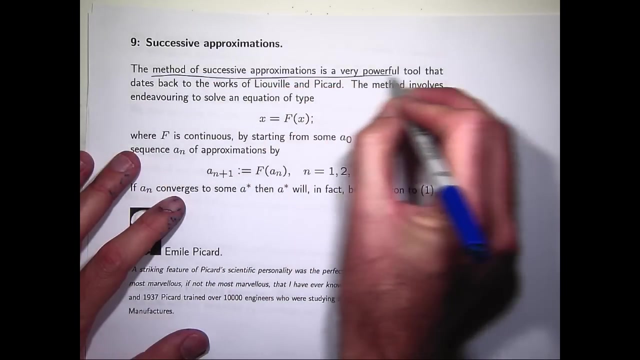 And in fact, I use this method in my own research from time to time. Oh, yeah, yeah, yeah, yep, yep, I've only got two slides to go. Okay, Now, now you may have heard of mathematicians. 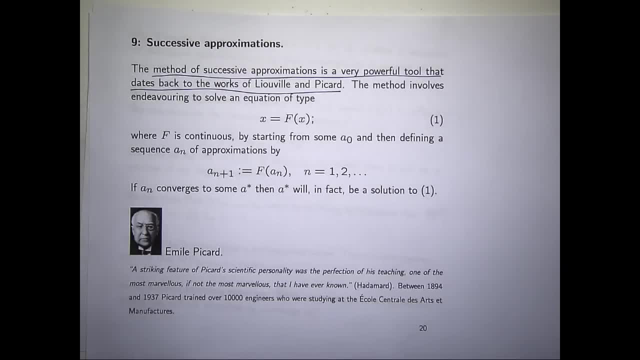 by the name of Picard and Louisville. okay, French mathematicians Very powerful. I love reading some of their work. Now they introduced a sequential way of approximating solutions of equations, So suppose we have an equation of this kind. 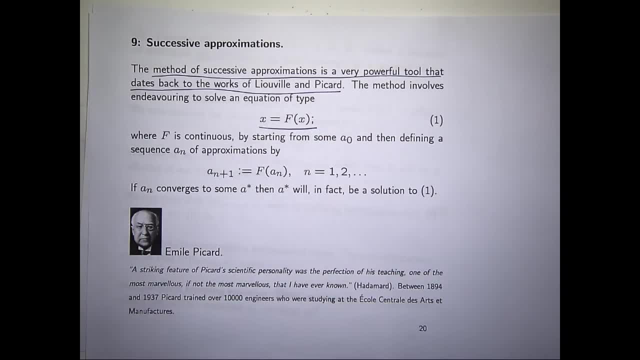 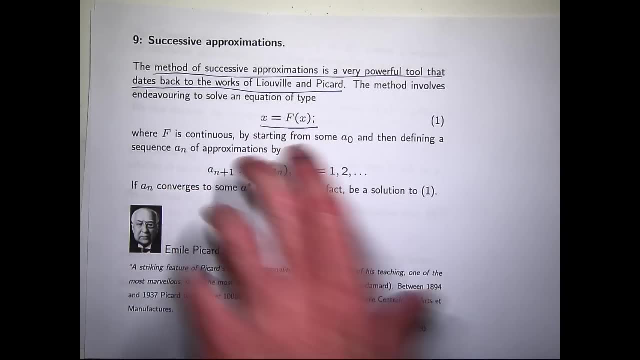 where f is some continuous function. Okay, Okay, This kind of problem it's known as a fixed point problem. Okay, So any x satisfying equation one is called a fixed point of the operator f. Now, if f is continuous, 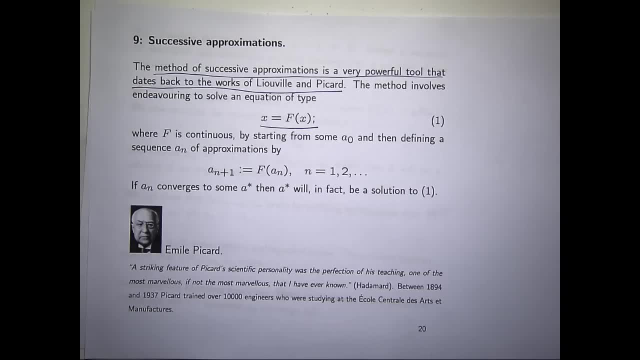 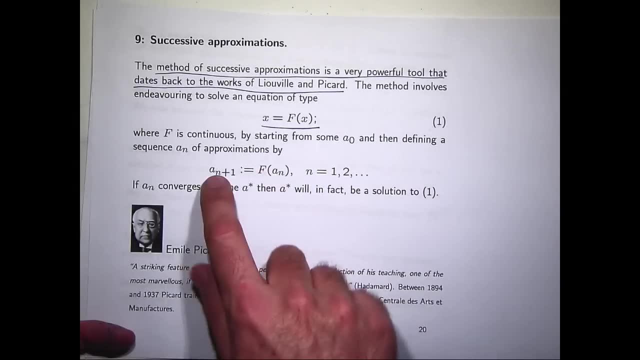 the method is as follows: You start with some value, a sub naught, and then you define a recursive representation for your sequence. a sub n- Okay. A sub n through the f here, Okay, Now, if f is continuous. if f is continuous. 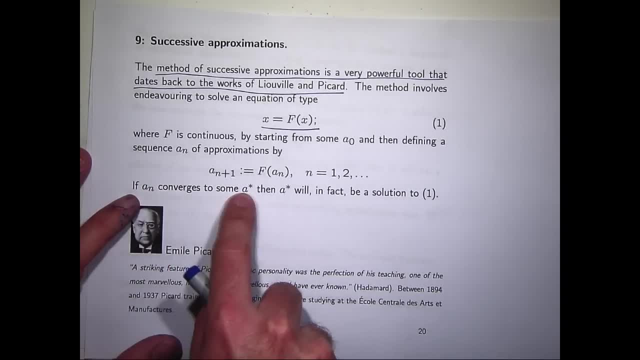 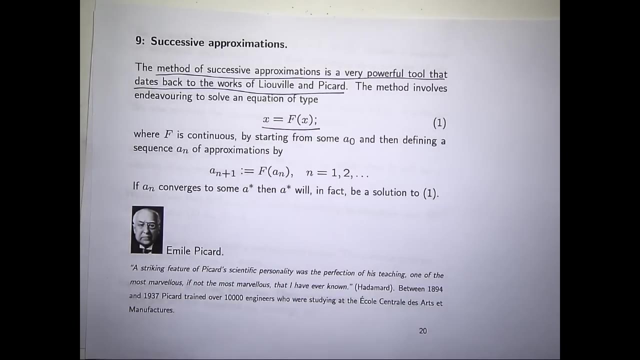 then and the a sub n converges to some limit- a star- then actually, if you take limits here and here, you'll get a star equals f of a star. So that means that a star, the limit will be a fixed point of f. 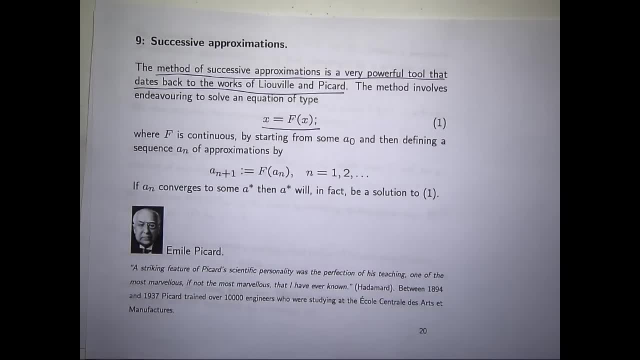 or a solution to the equation one. Okay, Now, that may not seem like much, but that method has been used over and, over, and, over and over again. Okay, It seems pretty simple, but it's really effective. Okay, So in one sense,